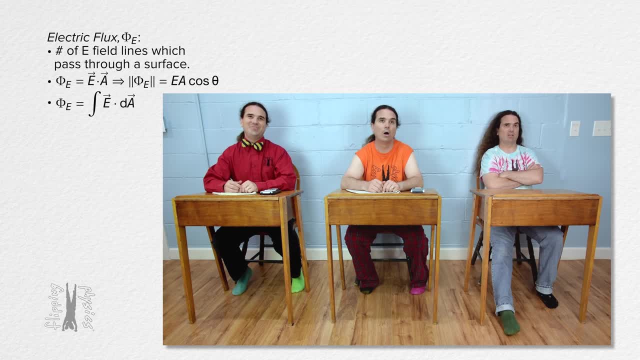 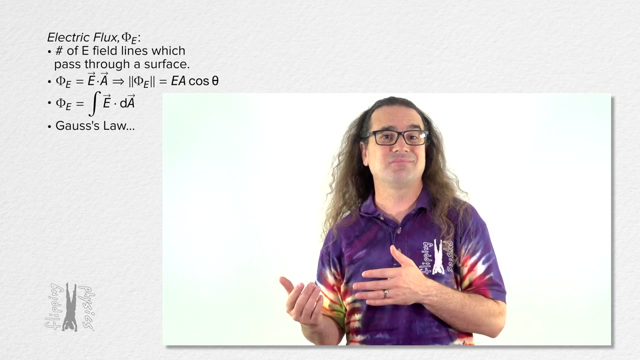 electric flux is that it equals the integral of the dot product of the electric field vector and the infinitesimal area vector dA. And I think Gauss's Law is in there somewhere. That is all correct. And Bo, yes, Gauss's Law is in there somewhere. 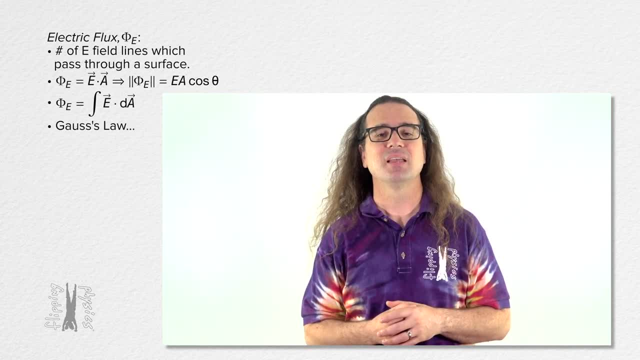 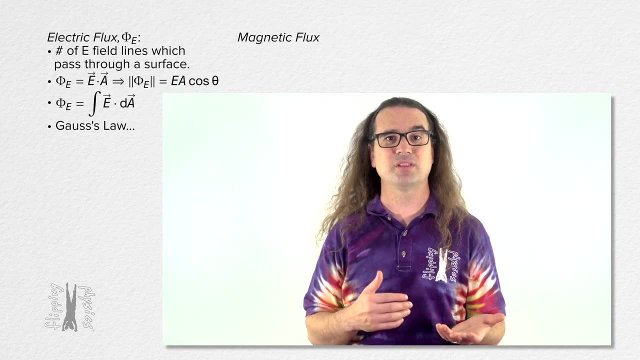 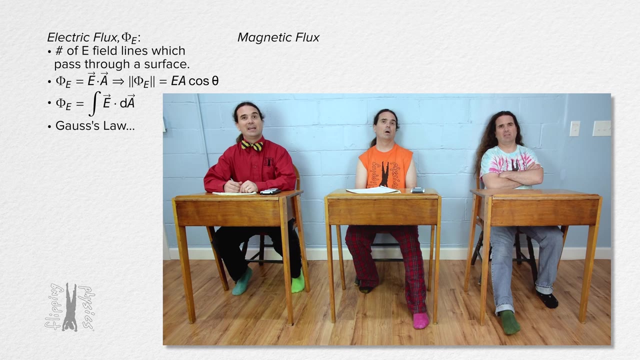 We will review that soon enough, However, not yet. Magnetic flux is pretty much what y'all just said, for electric flux only replace electric field with magnetic flux. So please say that all again, only for magnetic flux. Magnetic flux is like the measure of the number of magnetic field lines which pass through a surface. 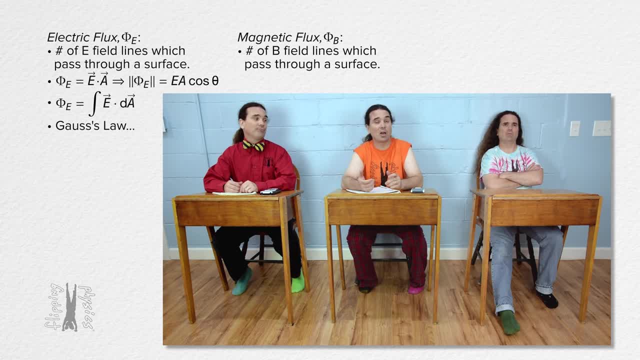 right Yep. And the symbol for magnetic flux is an uppercase phi with a subscript of capital B. And when the magnetic field is uniform and the surface is a two-dimensional plane, magnetic flux equals the dot product of the magnetic field vector and the area vector, or. 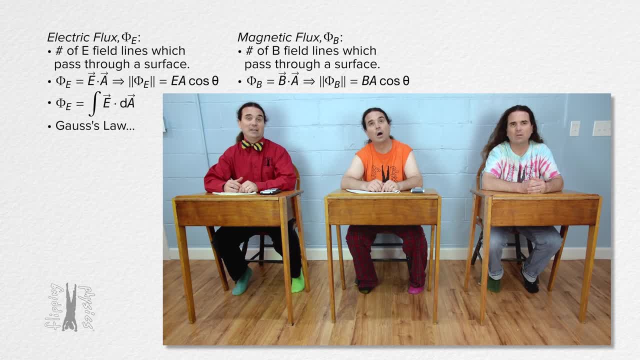 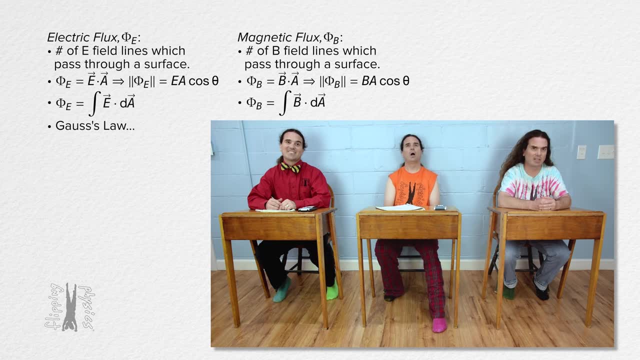 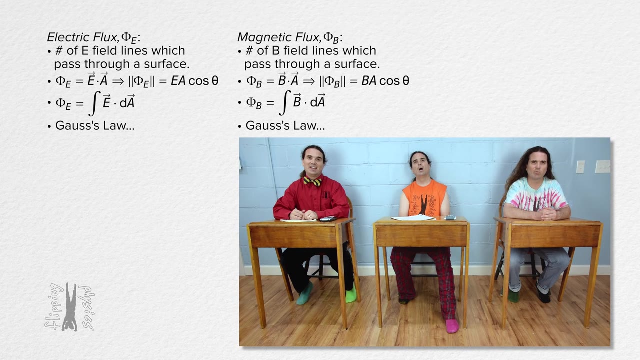 the magnetic field times, area times. the cosine of the angle between those two vectors And the more general equation for magnetic flux is that it equals the integral of the dot product of the magnetic field vector and the infinitesimal area vector dA. And I think Gauss's Law is in there somewhere. Everything you just said is correct, Thanks. 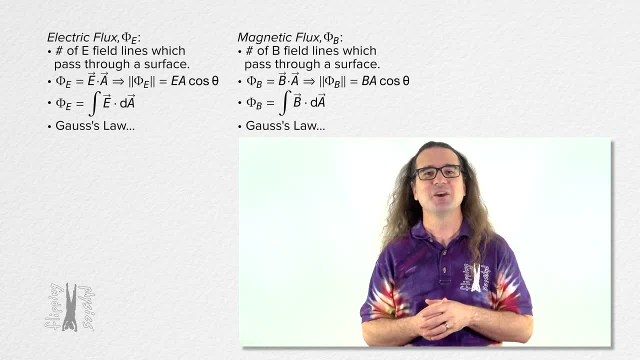 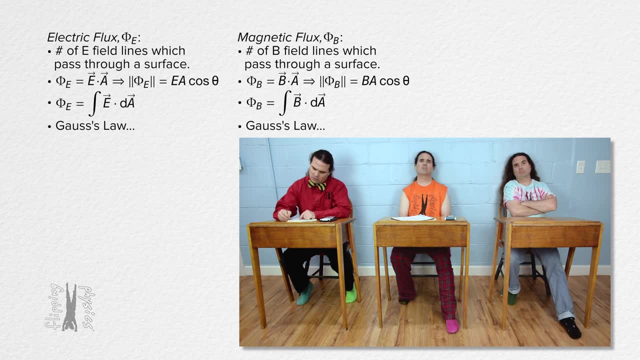 Anytime, Mr Payton. Sure, you are welcome. Bobby, what are the units for magnetic flux? The units for magnetic flux are: well, the units for magnetic field are Teslas and area just meters squared, So Teslas times square meters. 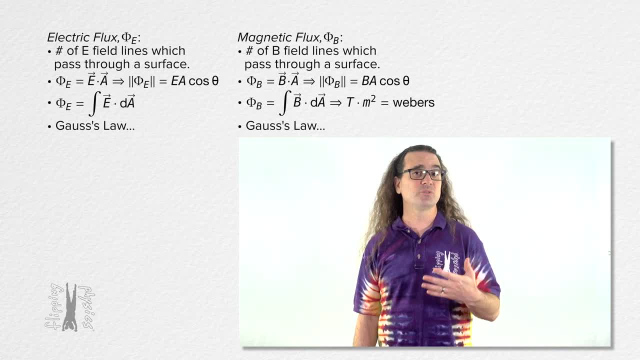 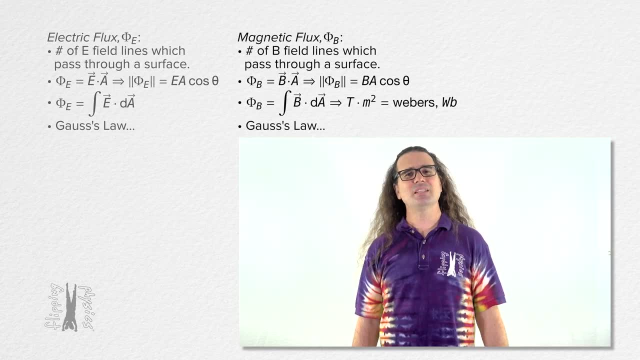 Correct, Bobby, And those are called webers And we use wb with an uppercase w as the shorthand notation for webers. Webers, Yep, Webers. Let's look at a basic example. Let's say we have a singular circular loop of wire with current passing through it. 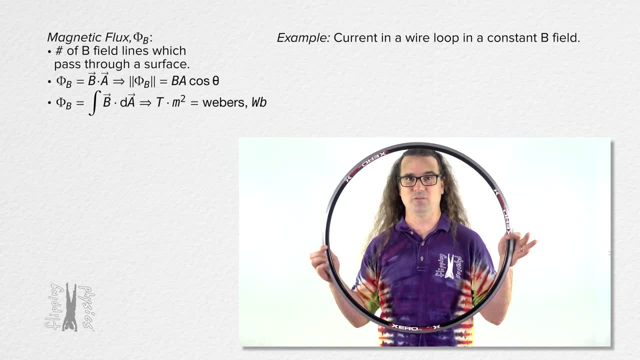 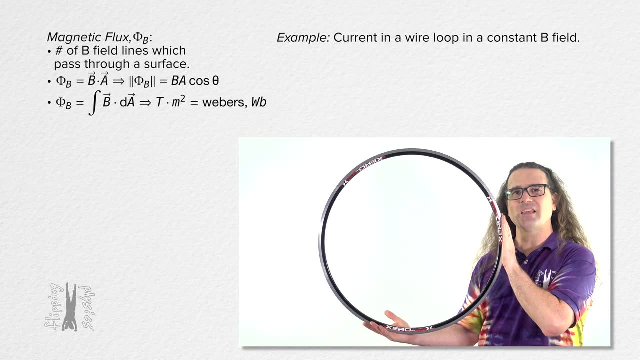 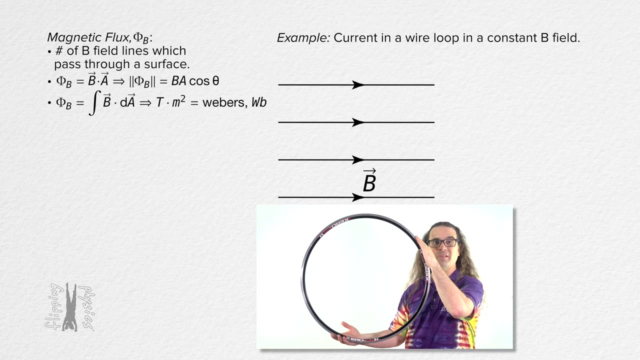 To give us a visual, please observe this bike wheel rim. Imagine the bike wheel rim is a single wire with current passing through it. For this example, let's have a uniform magnetic field acting to the right. Let's have the rim oriented such that the plane of the loop is horizontal, and let's 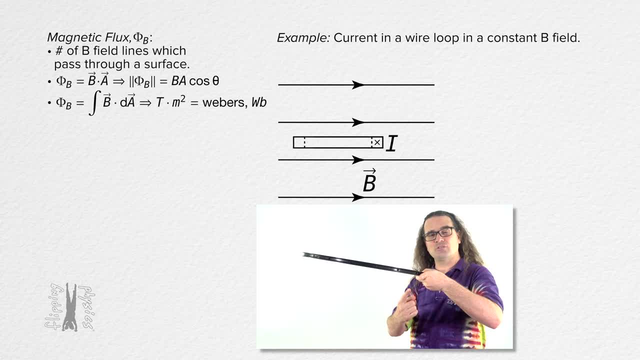 have current going through the loop such that it is going into the screen on the right side of the wire loop and going out of the screen on the left side of the wire loop To determine the direction of the area vector class. what handy tool do you think we use? 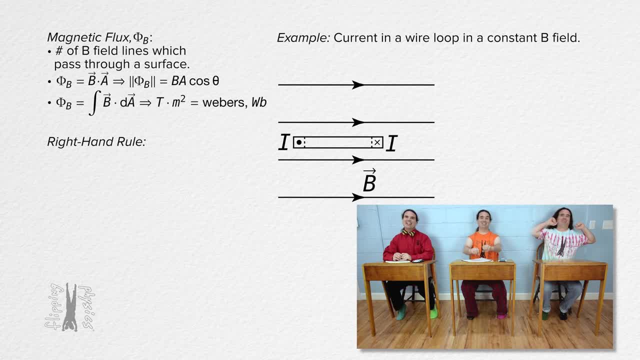 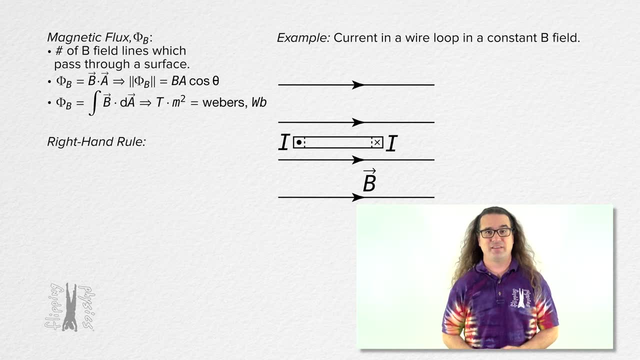 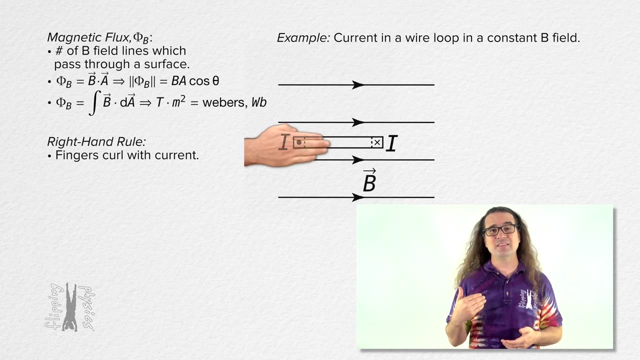 The right-hand rule to find the direction of the area vector corresponding to a loop that can carry current is similar to the right-hand rule for angular velocity. Fingers curl in the direction we choose for positive current in the loop And thumb points in the direction of the area vector. 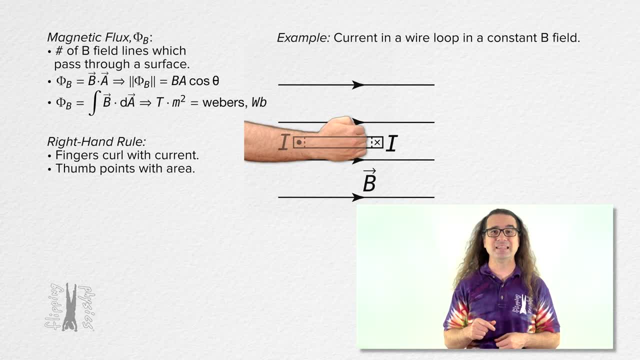 In other words, the area vector caused by the current in the loop in this example is up towards the top. Now that we have the area vector direction, you should be able to see that the angle between the magnetic field and the area vector is 90 degrees. 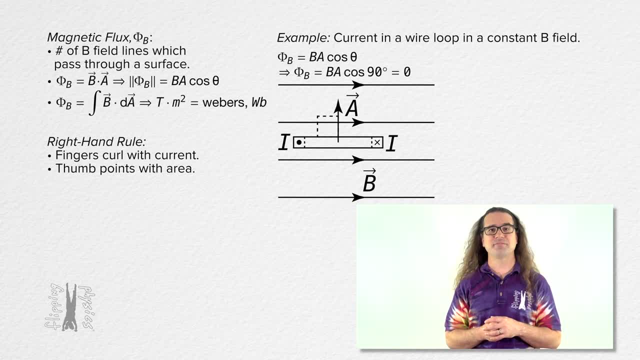 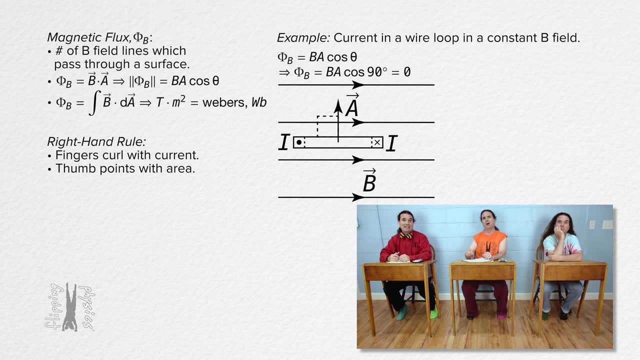 The cosine of 90 degrees is zero. Therefore the magnetic flux through this loop, in this magnetic field, is zero right now. That makes sense because magnetic flux is a measure of the number of magnetic field lines which pass through the loop and because the plane of the loop is parallel to the magnetic 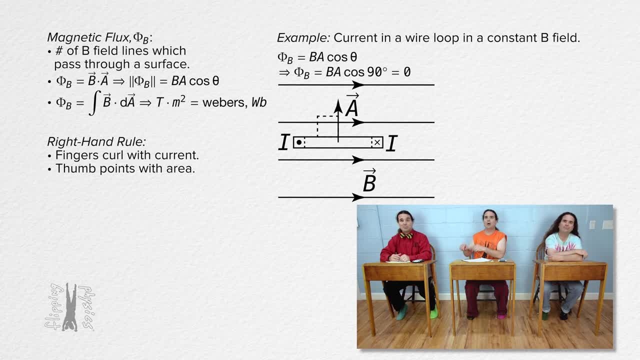 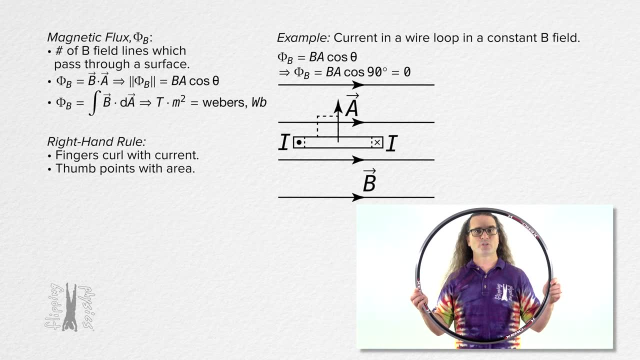 field, zero magnetic field lines pass through the loop. In other words, there is zero magnetic flux through the loop. Right, Mr P? Exactly, Billy. Let's turn the bike rim, which represents a wire loop, so the plane of the loop is vertical. 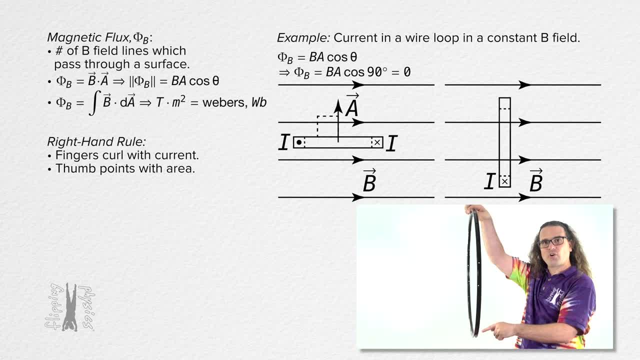 with current going into the screen on the bottom and current going out of the screen on the top of the loop. Bobby, tell me what you know about the magnetic flux passing through the wire loop in this example. Sure Well, we start with the right-hand rule. 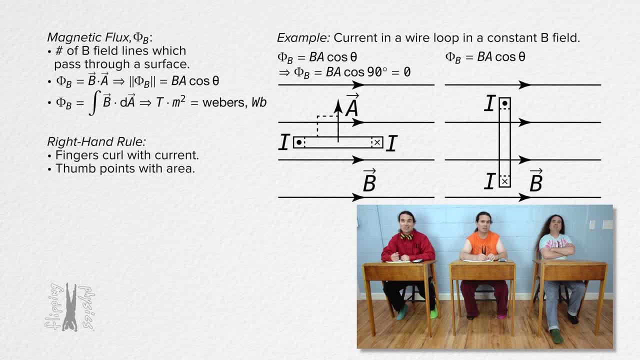 We use the right-hand rule to determine the direction of the area vector caused by the current-carrying loop. Curl our fingers in the direction of the current and our thumb points to the right. So the area vector is to the right. The magnetic field is also to the right. 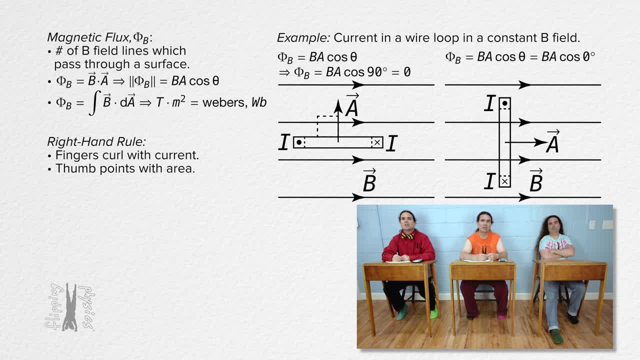 The angle here between the magnetic field and the area vector is zero and the cosine of zero degrees equals one. So this orientation gives the maximum magnetic flux through the current-carrying loop. At any other angle, Well, the cosine of the angle will give a value less than one and give a smaller magnetic 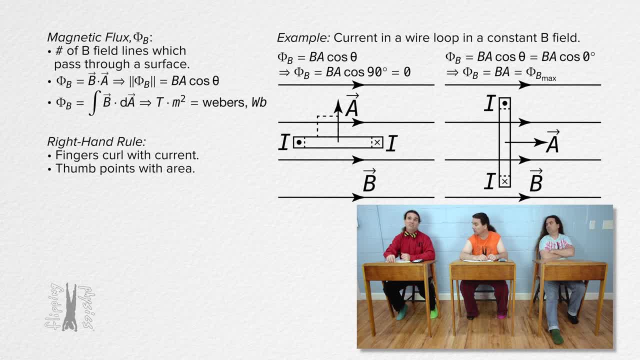 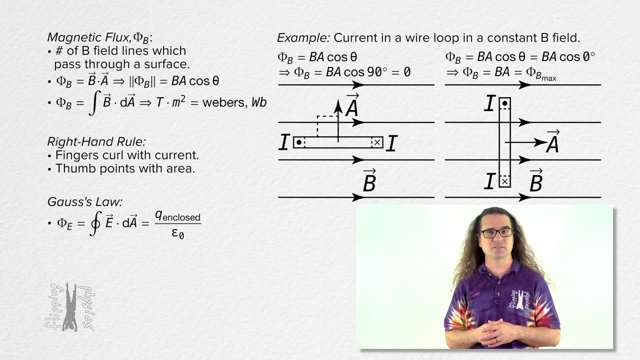 flux value. That makes sense because if we turn the loop, even a little bit, the number of magnetic field lines which pass through the loop will be decreased, which shows that the magnetic flux is decreased. Cool, Agreed. Now, if you recall, Gauss's Law has to do with electric flux. 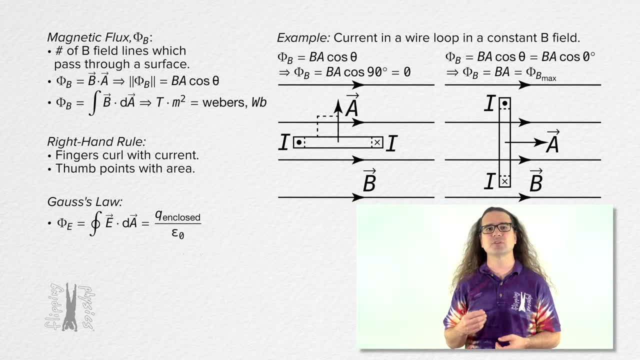 Gauss's Law states that the electric flux through a closed surface equals the closed surface integral of the dot product of electric flux. Cool, That's what I'm going to figure out right now. It's called the magnetic flux through a closed surface integral. 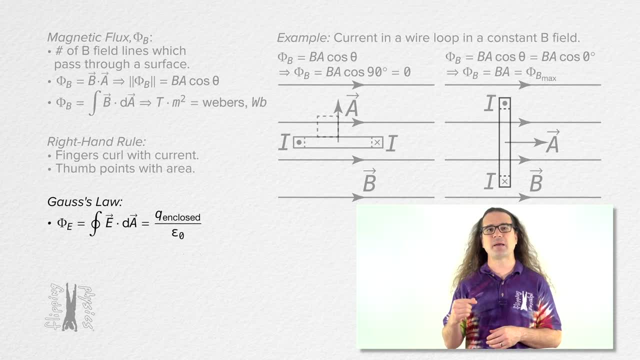 There's not any reason to rule out the magnetic flux through a closed surface integral, which is the charge of the dot product of magnetic field and the area vector. This is just a 1 to 1 test, So 1 to 1 number must be equal to the magnetic flux through a closed surface integral of. 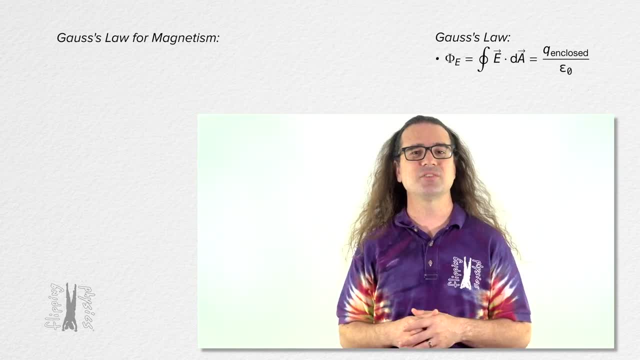 the dot product of electric flux. Well, if I'm done with this, I'm going to run a test to see how I can determine the magnetic flux through a closed surface integral of electric flux. The first level of my limit is 1 to 1.. You can calculate the magnetic flux of electric flux through a closed surface integral by adding up the dot product of magnetic flux by dividing it by the area vector. If I have these two numbers and add up the series of factors, I can get 1 to 1.. 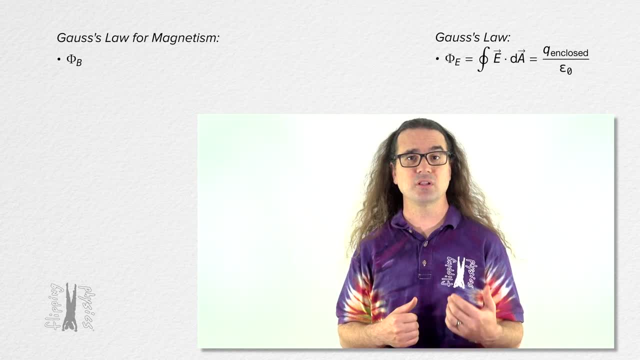 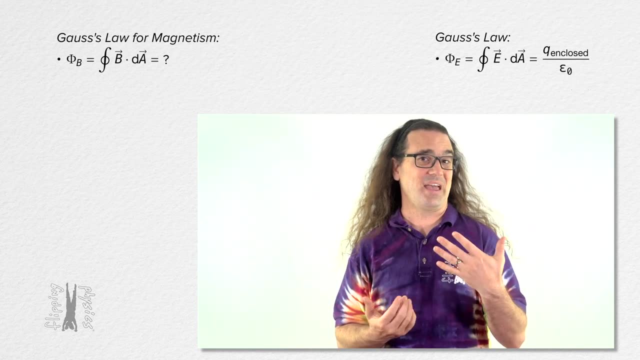 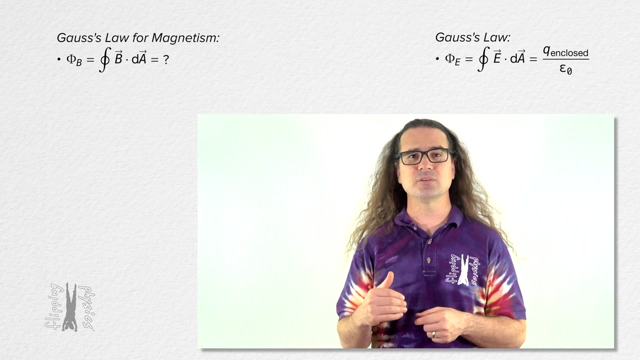 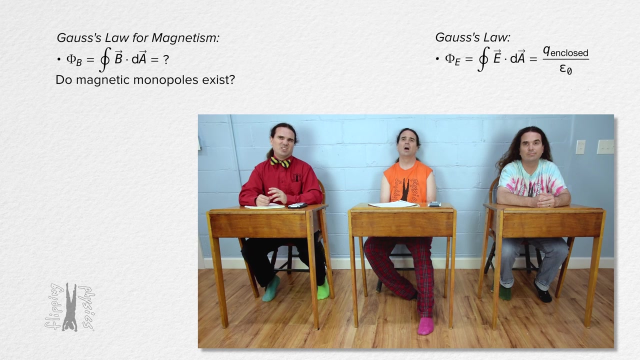 How do you do that flux through a closed surface equals? remind me, Billy, do magnetic monopoles exist? Do magnetic monopoles exist? In other words, can you have a north magnetic pole without also having a south magnetic pole connected to it? 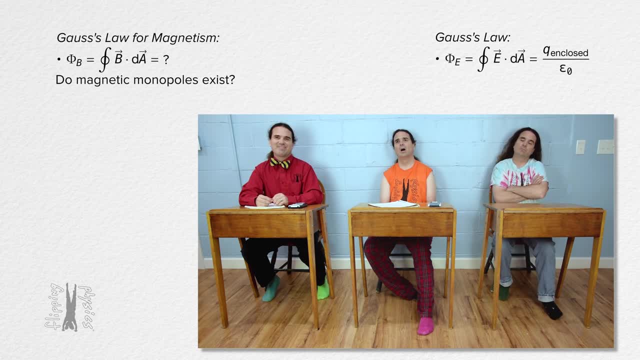 Or a south magnetic pole without also having a north magnetic pole connected to it. Okay, yeah, I remember this. A magnetic monopole has never been found in nature or in a man-made experiment, meaning we cannot prove magnetic monopoles do not exist. however, one has never been found, so 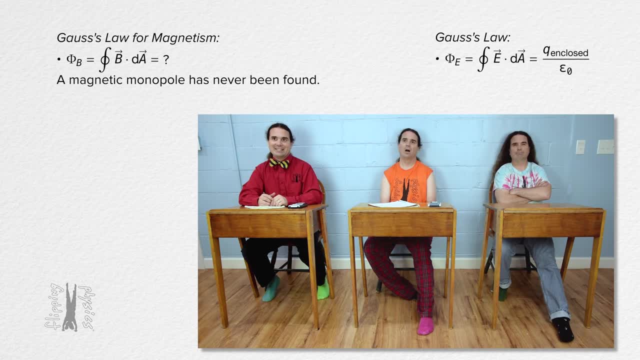 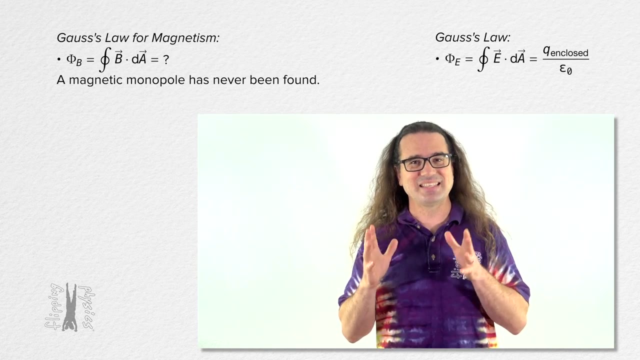 at this point we assume that magnetic monopoles do not exist, And someday, if we find a magnetic monopole, it will throw into question everything we use to describe how our universe works. Nice, Yeah, A bit dramatic, but yes. 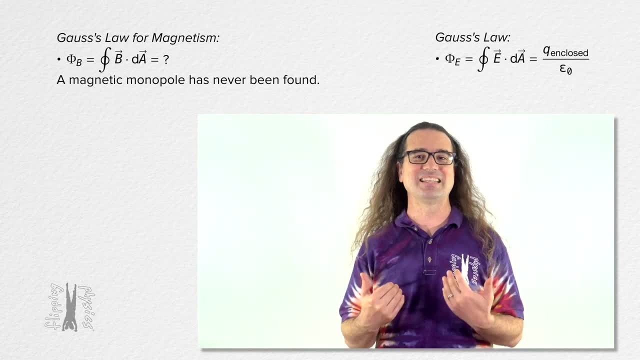 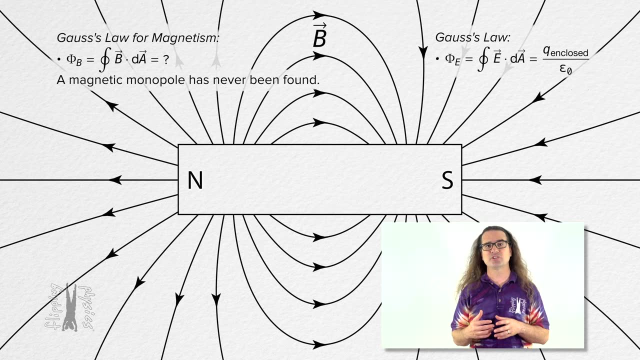 It is true that magnetic monopoles have never been found in nature. To recall what that means for magnetic fields, let's put an illustration of a magnetic field which surrounds a dipole. magnet Bo. remind me what the fact that magnetic monopoles have never been found in nature. 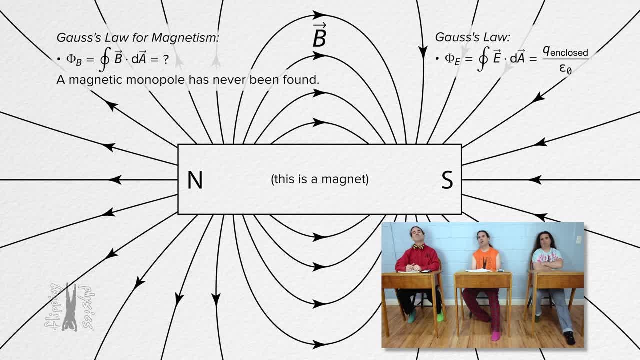 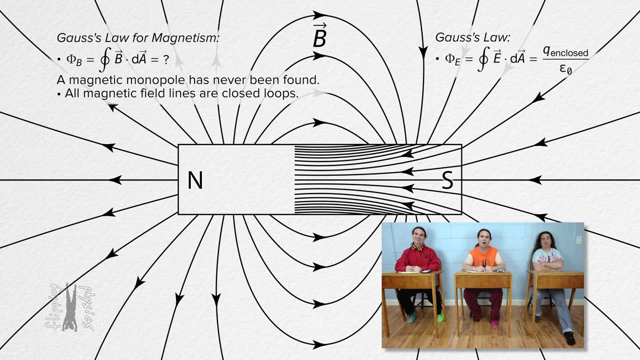 means for magnetic fields? Sure, Because magnetic poles always come in pairs, magnetic field lines are always closed loops And that means that inside the magnet the magnetic field lines go from south to north to complete the closed loops. Correct, Bo, Every magnetic field line is a closed loop. 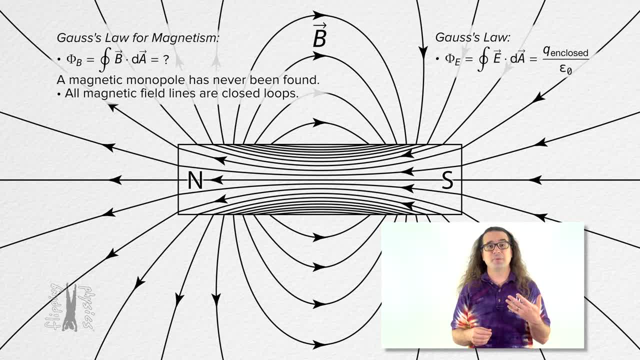 Most of the magnetic field line loops in this illustration actually reach beyond the area of this screen but realize they are still loops, just very large loops. But let's return back to why we have this illustration on the screen. We are trying to determine what the magnetic flux through a closed surface equals. 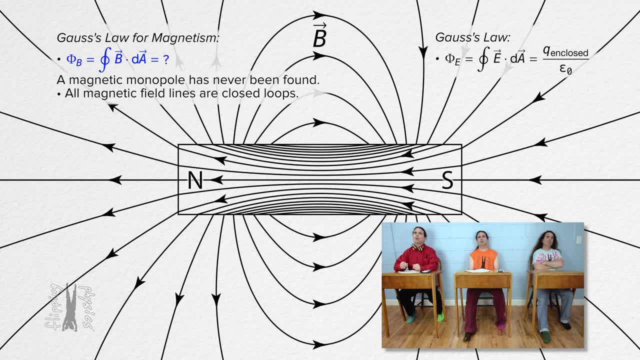 Bobby, what do you think? Well, I guess we should draw a Gaussian surface and see what we see. Let's start with a sphere for a Gaussian surface. Ah, Magnetic flux is the measure of the number of magnetic field lines which pass through. 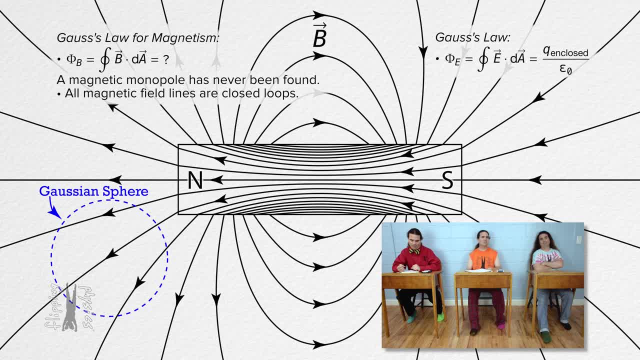 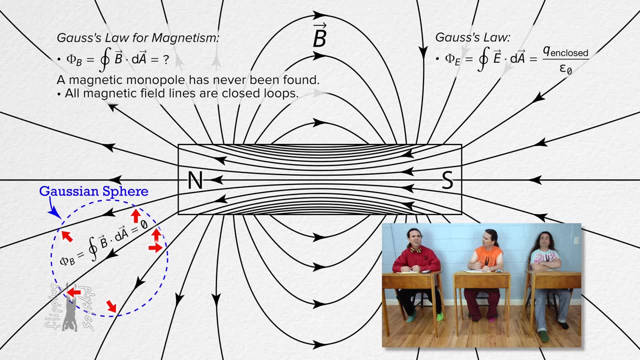 a surface. Right You can see that every magnetic field line which goes into the magnetic field line is a Gaussian surface and the magnetic field line which goes out of the-into the Gaussian surface also comes out of the Gaussian surface. so the net magnetic flux through this Gaussian 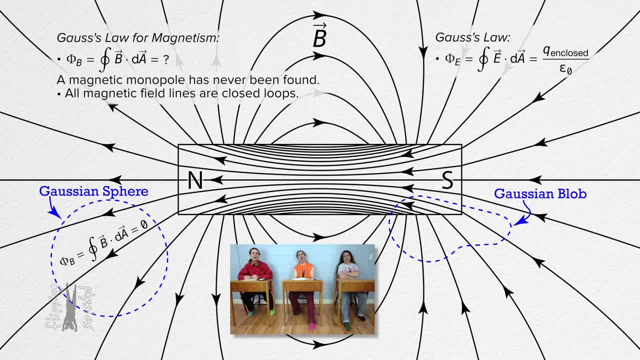 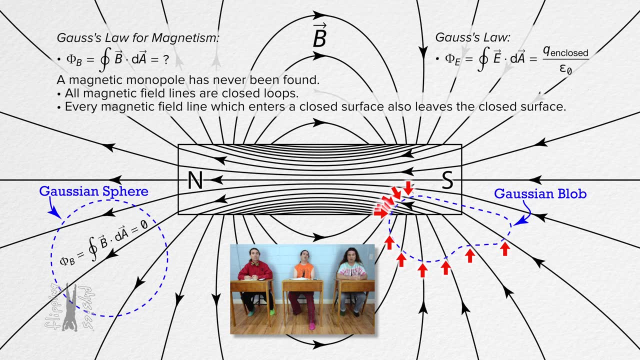 sphere equals zero. Is that always true? …if you draw a randomly shaped Gaussian surface, even with part of the Gaussian surface inside the magnetic dipole, you can see that every magnetic field line which goes into the Gaussian surface also comes out of the Gaussian surface. 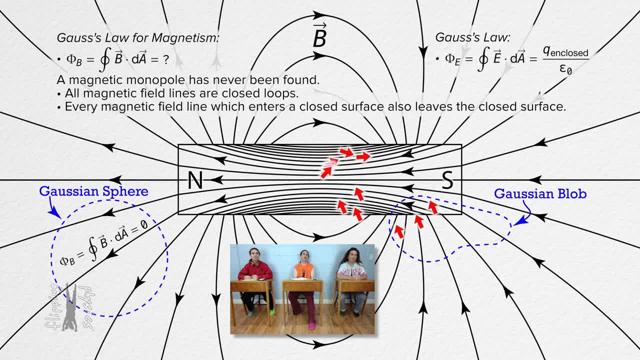 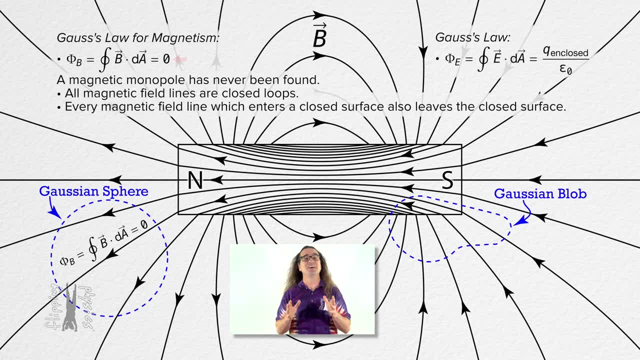 closed loops. the magnetic flux through a closed surface always equals zero. Am I right, Mr P Bo, that is absolutely correct. Thanks, You are welcome. Please realize this equation is specifically called Gauss's Law for Magnetism and is the 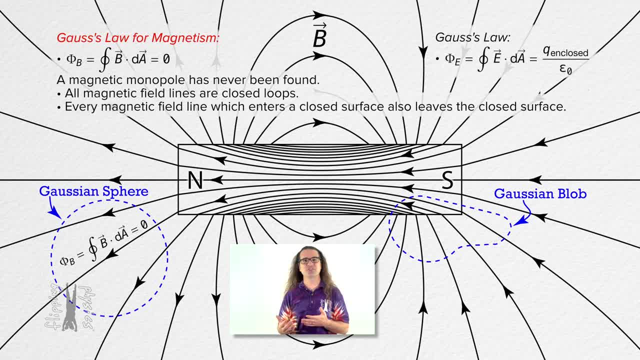 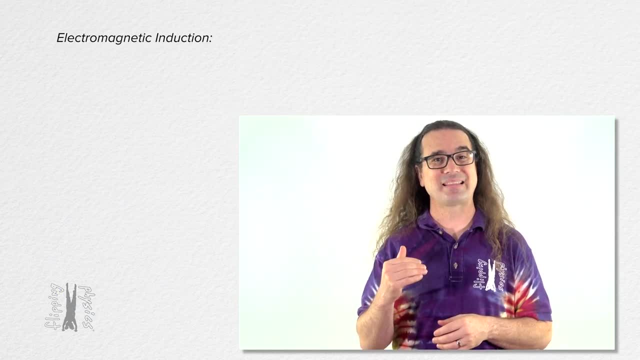 second of Maxwell's equations, which are a collection of equations which fully describe electromagnetism. We have now talked about three out of the four of Maxwell's equations. Almost there, So close, Yeah. Now we can begin talking about electromagnetic induction. We have already. 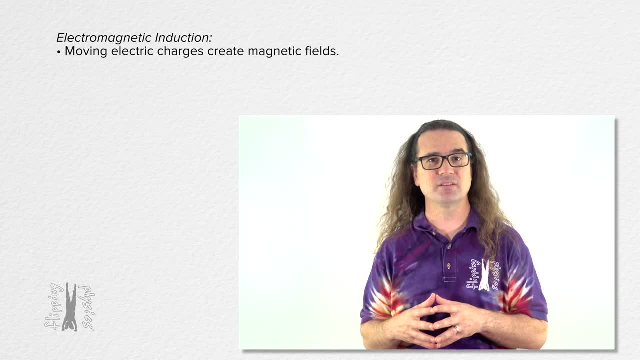 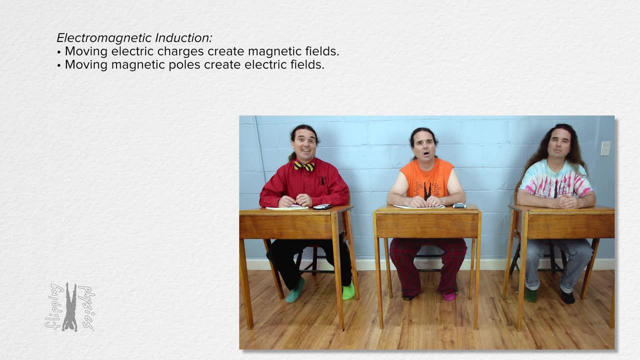 discussed that moving electric charges create magnetic fields. It really should be no surprise then that moving magnetic poles create electric fields. Wait, So moving electric charges create magnetic fields, which cause magnetic forces on magnetic poles, Which can move magnetic poles, and moving magnetic poles create electric. 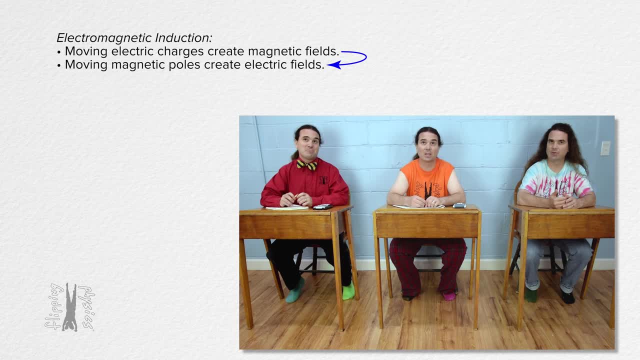 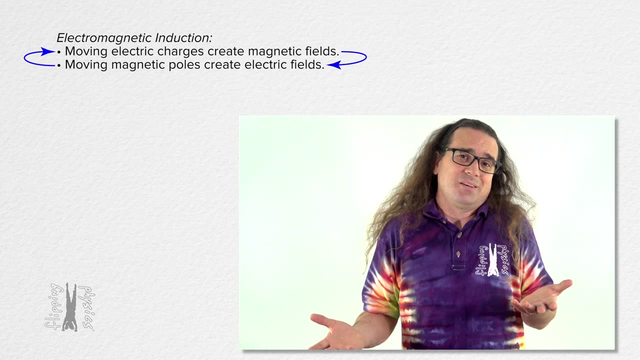 fields Which cause electric forces on electric charges, Which can move electric charges, and moving electric charges create magnetic fields, Which is what I just said. Yeah, Exactly, Which is basically why an electromagnetic wave can self-propagate, But we're getting ahead. 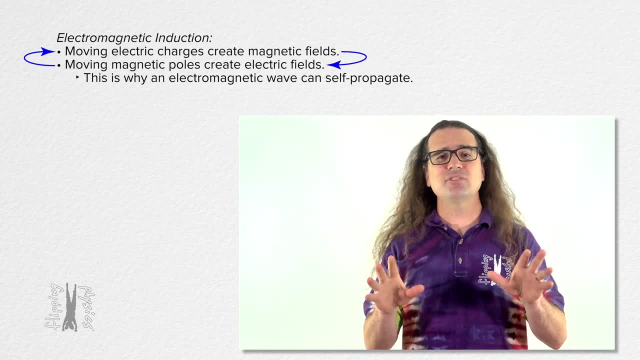 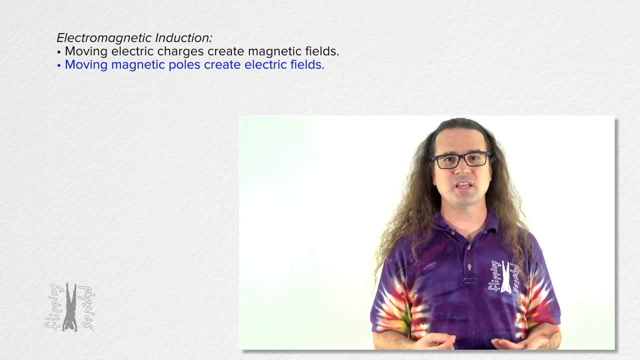 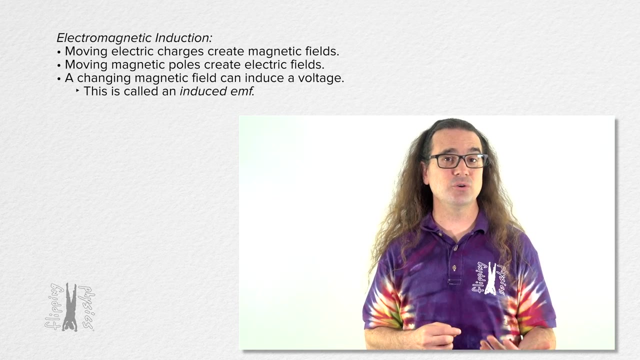 of ourselves. with that bit of logic, Let's just return to the fact that moving magnetic poles create electric fields. When a magnetic field changes over time, this can induce the same outcome as an electric potential difference, and it is called an induced EMF. An induced EMF can cause charge. 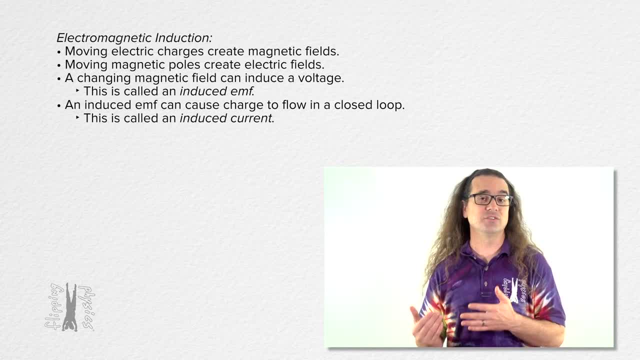 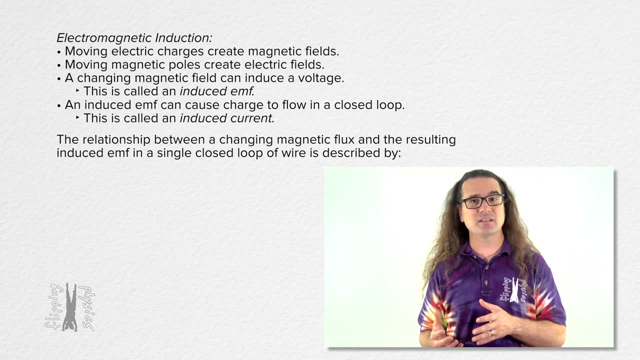 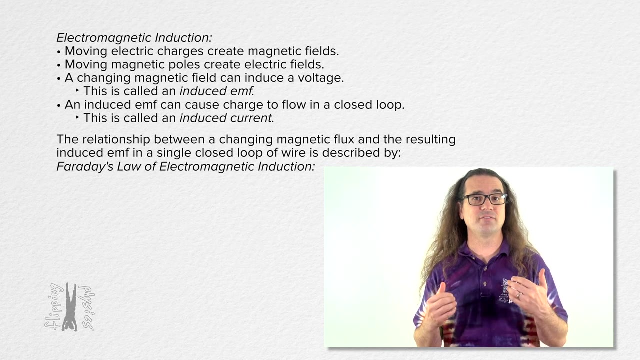 to flow in a closed loop of wire, which is called an induced current. More specifically, the relationship is between a changing magnetic flux and the resulting induced EMF in a single closed loop of wire and is described by Faraday's Law of Electromagnetic Induction, which states that the 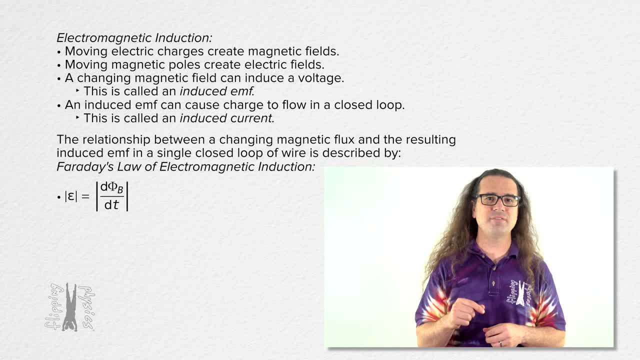 absolute value of the induced EMF is the absolute value of the induced EMF. The absolute value of the induced EMF is the absolute value of the induced EMF. The absolute value of the induced EMF is the equals, the derivative of magnetic flux with respect to time or the time rate of change of. 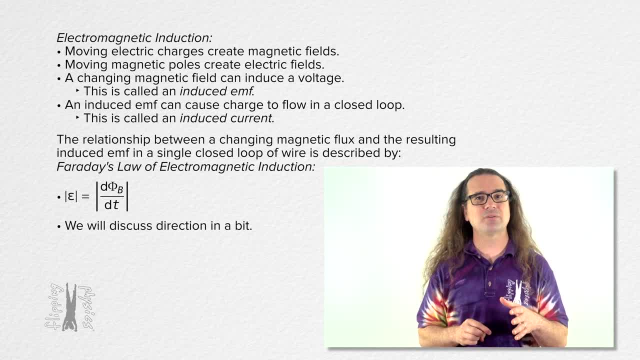 magnetic flux. In a bit we will talk about the direction of the induced EMF and induced current caused by the changing magnetic flux. However, for now let's only concern ourselves with the absolute value of the induced EMF. What does EMF stand for? 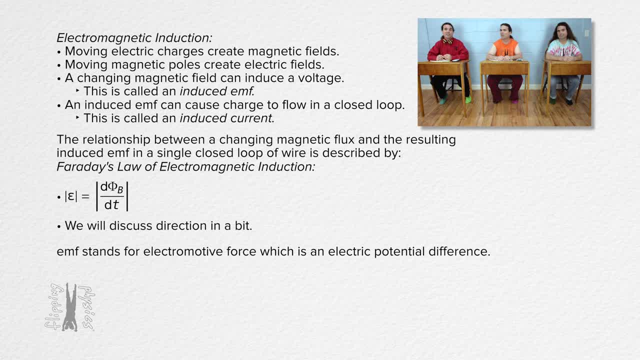 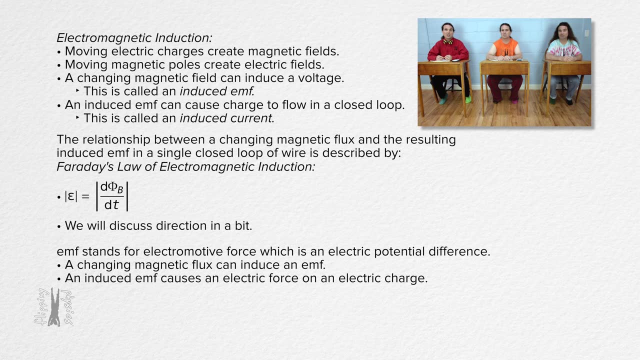 Electromotive force, Which is an electric potential difference. But we just learned that a changing magnetic flux can induce an electromotive force, Which is an electric potential difference, And that induced EMF causes an electric force on an electric charge. Maybe that is why it is called an electromotive force. 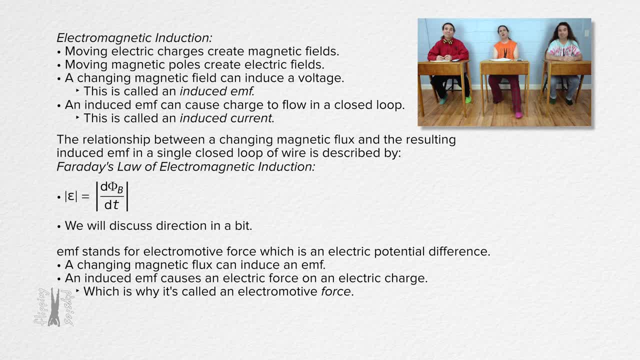 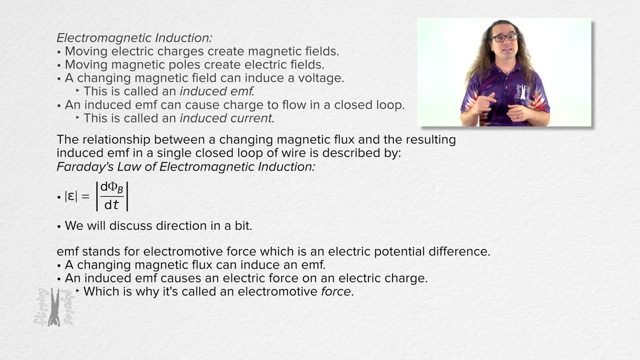 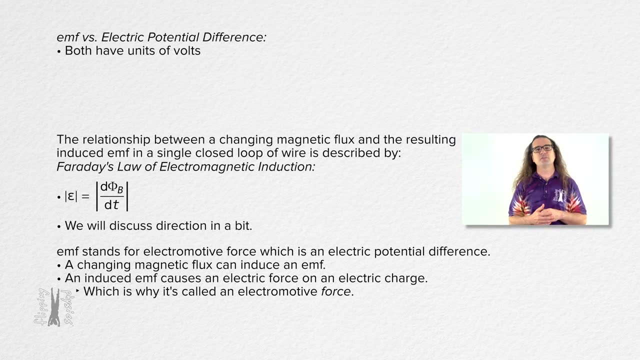 That actually makes a lot of sense. Yeah, Correct, Bobby. That is why it is called an electromotive force. Nice work everyone. Billy, I would like to discuss a point you made comparing EMF and electric potential difference. Both have units of volts and 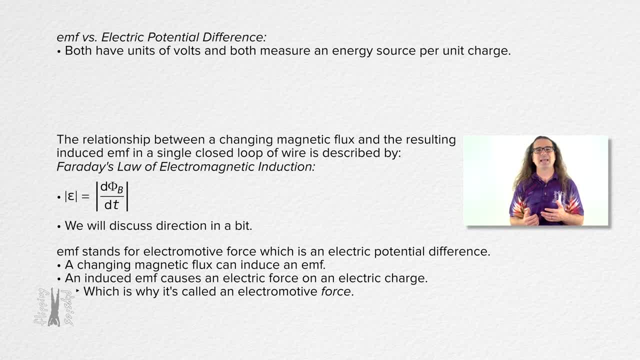 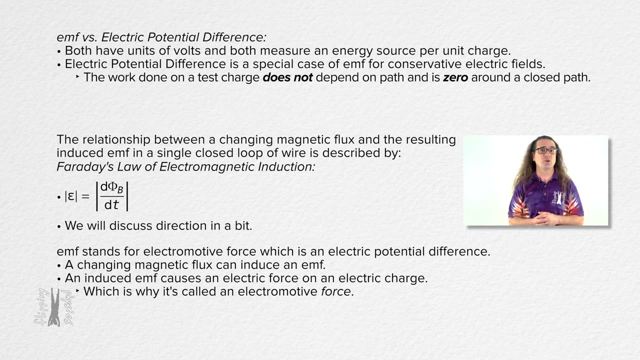 both measure an energy source per unit charge. However, electric potential difference is a special case of EMF for conservative electric fields And the difference in electric potential works as a shortcut for determining work done on a test charge. When a changing magnetic flux induces an EMF, the field is not conservative. the work done on a 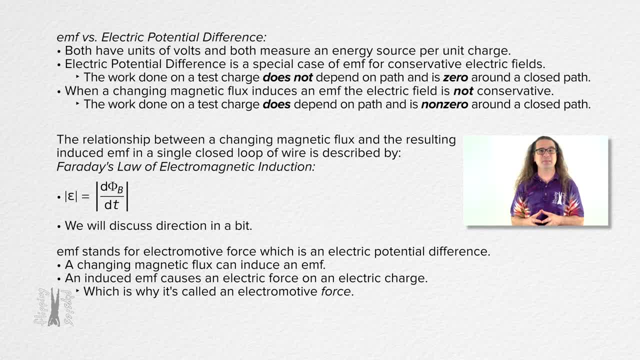 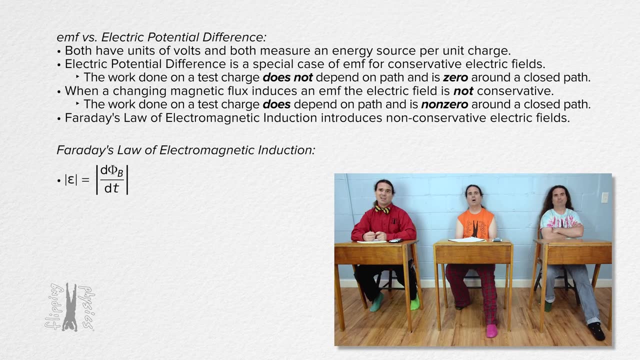 a test charge will depend on the path and will no longer be zero around a closed path. Faraday's Law of Induction induces non-conservative electric fields where EMF is no longer as simple as a difference of electric potential across two points. Okay, back to Faraday's Law of Induction. 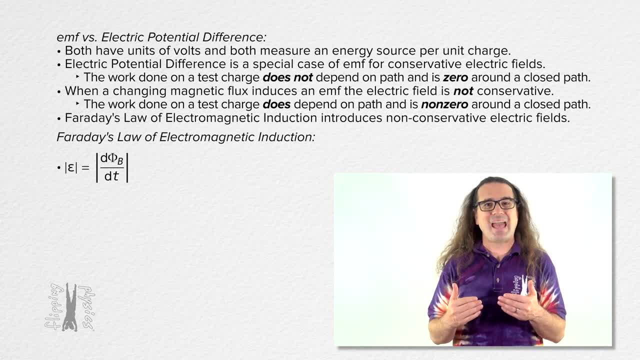 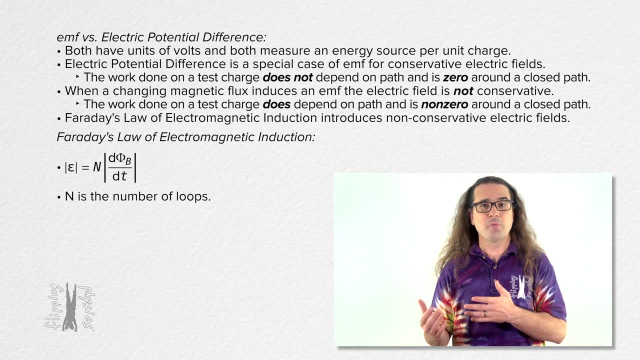 which I am going to expand on a bit. I'm going to add a capital N, which stands for the number of loops through which the magnetic flux is changing. We know magnetic flux equals the dot product of the magnetic field and the area vector of the loop through which the magnetic 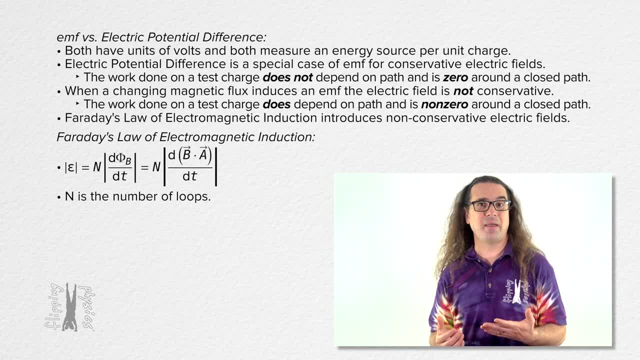 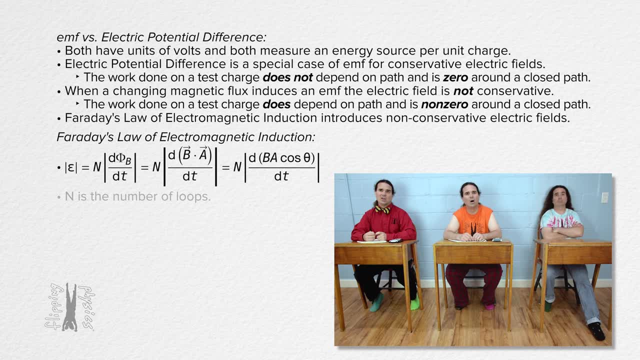 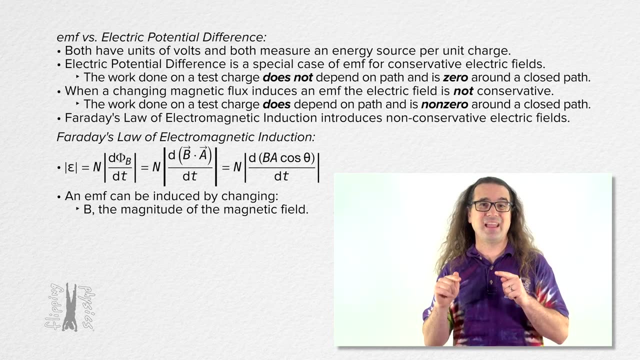 field is passing And the dot product is the same as the magnetic field times. the loop area times the cosine of the angle between those two vectors. Therefore, notice, an EMF can be induced by changing the magnitude of the magnetic field, the area enclosed by the loop. 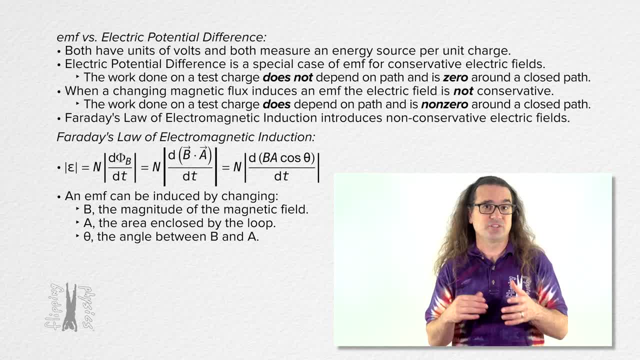 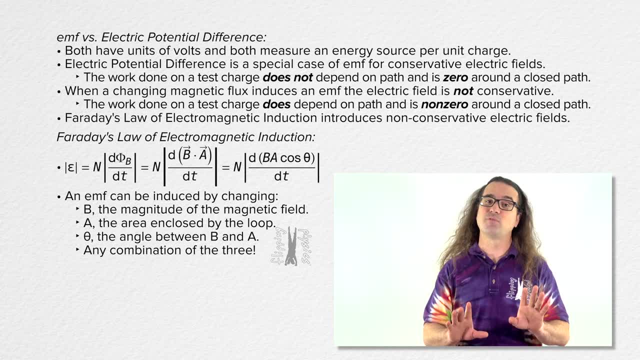 the angle of the magnetic field, the area enclosed by the loop between the magnetic field and the loop area which is theta in the equation, or, my personal favorite, any combination of the three. For example, if the only one of these three variables magnetic field, loop area and. 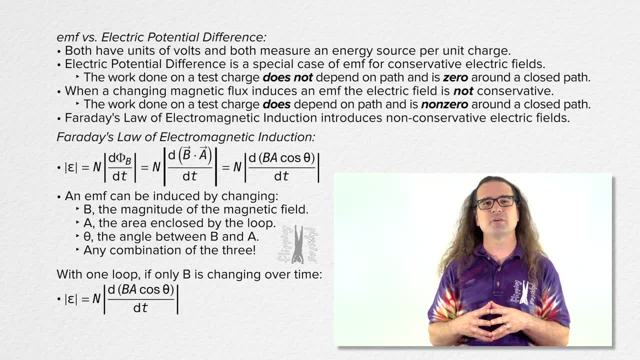 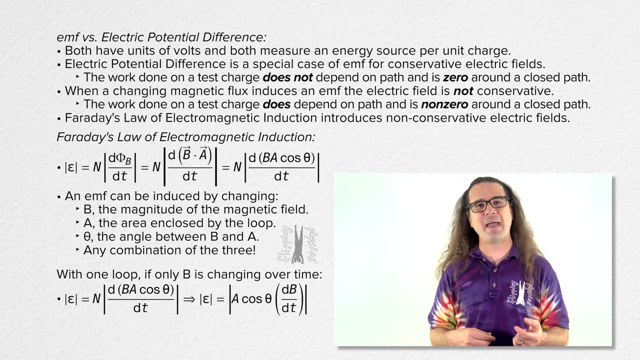 the angle between the two. if the only one of those three variables which is changing is the magnitude of the magnetic field, then the induced EMF through one loop of wire equals the magnitude of the loop area times the cosine of the angle between the area vector and the 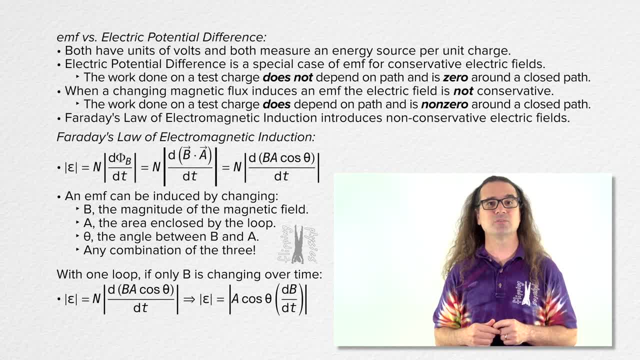 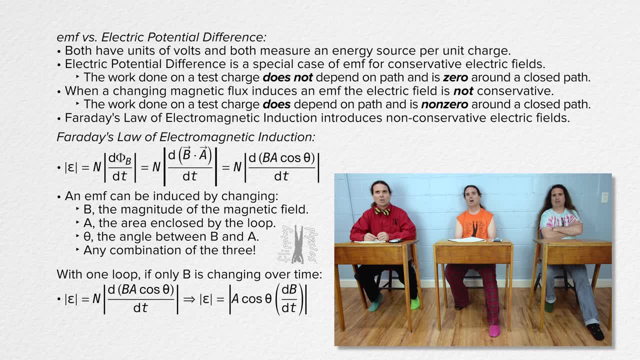 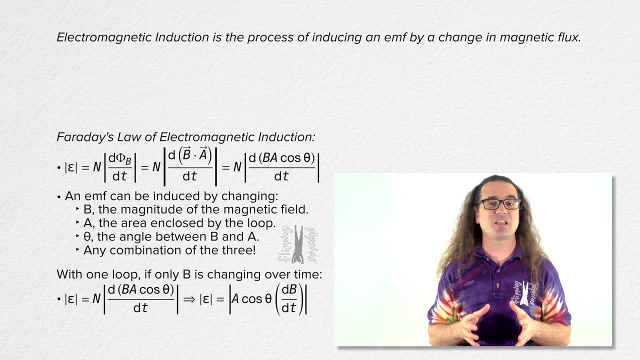 magnetic field vector times the derivative of the magnetic field with respect to time. That makes sense, Sure, Okay. But what is electromagnetic induction? I don't think we've actually defined that yet. Yeah, I can see that, Okay. Electromagnetic induction is the process of inducing an electromotive force by a change. 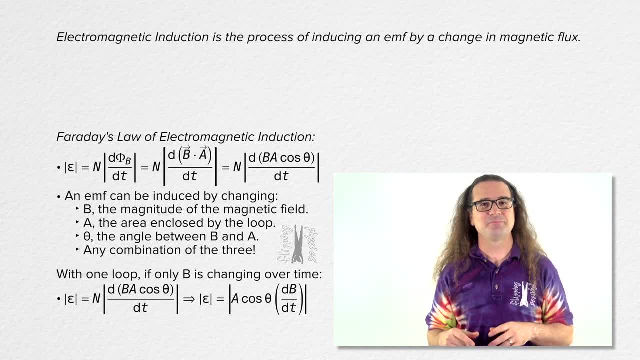 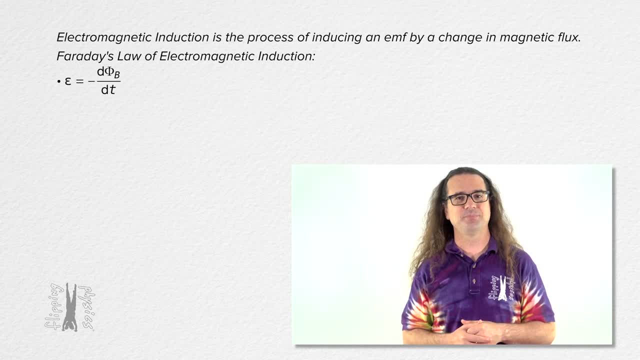 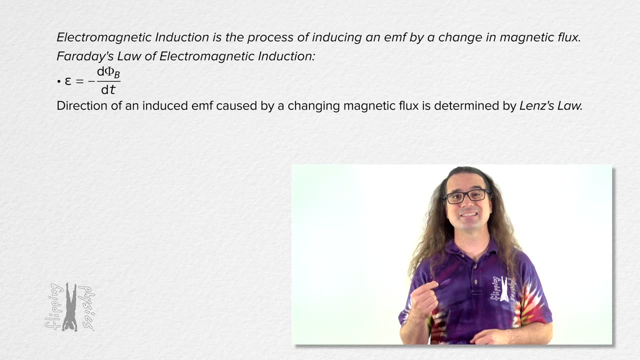 in magnetic flux. Thanks, Alright, Now we add direction to Faraday's Law by adding a negative sign and removing the absolute value. Believe it or not, the direction of the induced EMF caused by a changing magnetic flux is called Lenz's Law. 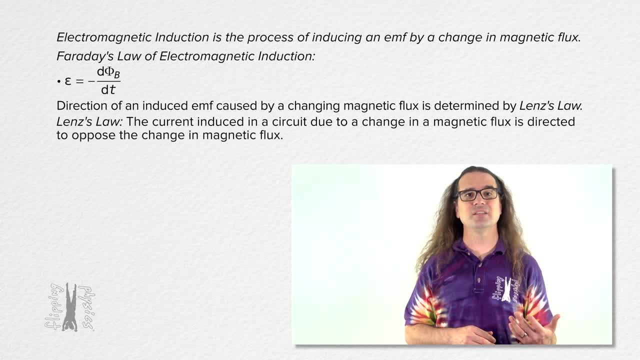 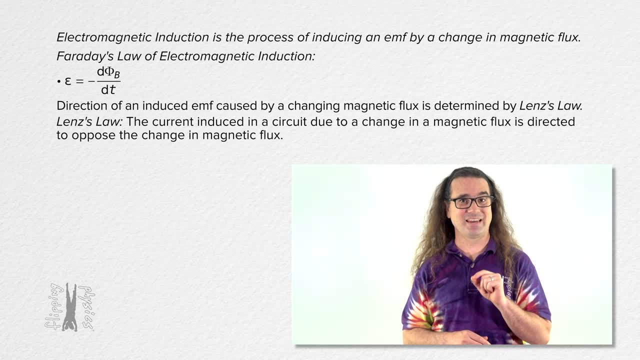 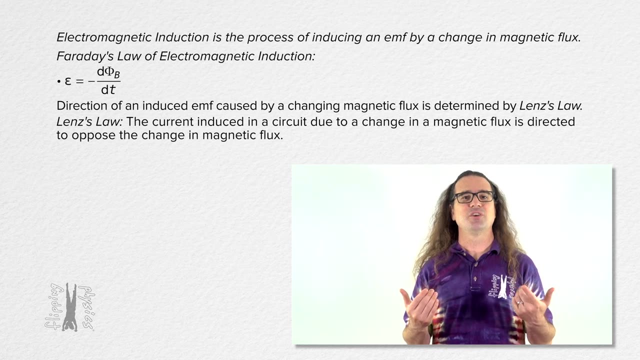 More specifically, Lenz's Law states that the current induced in a circuit due to a change in a magnetic flux is directed to oppose the change in magnetic flux. Wow, Yeah, To help us understand what that means. class to determine the direction of the induced. 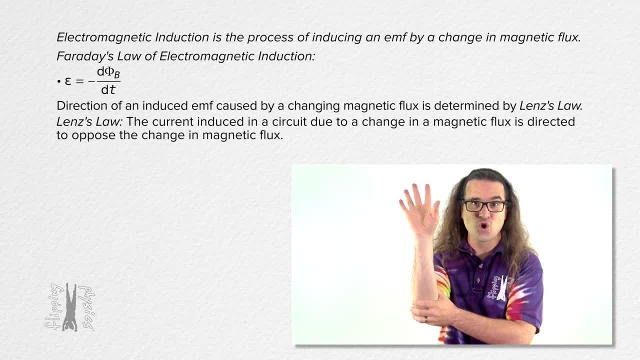 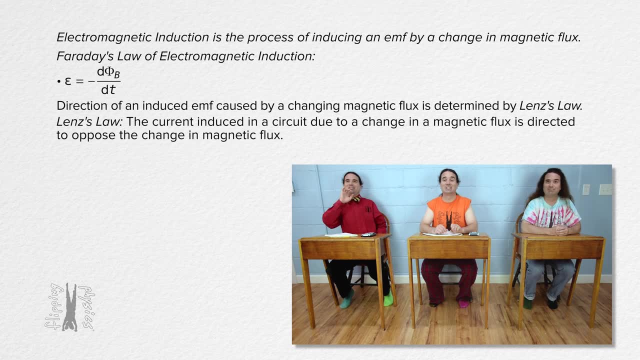 current in a loop caused by a change in magnetic flux. What handy tool do you think we use? The right-hand rule, Of course. Don't be too cool, Limber up And find your right hand. I feel like we already did this. 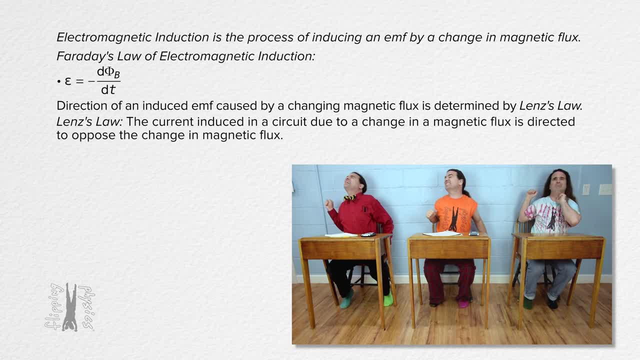 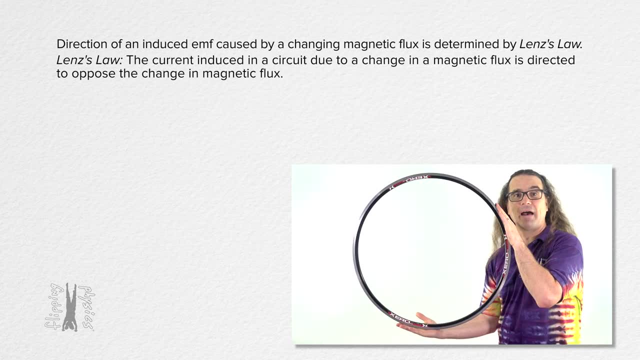 Did we, But it feels so good. Yeah, Alright, Here we go. Let's learn from doing examples. We have our wire loop and initially there is zero magnetic field inside the loop and therefore zero magnetic field within the loop. 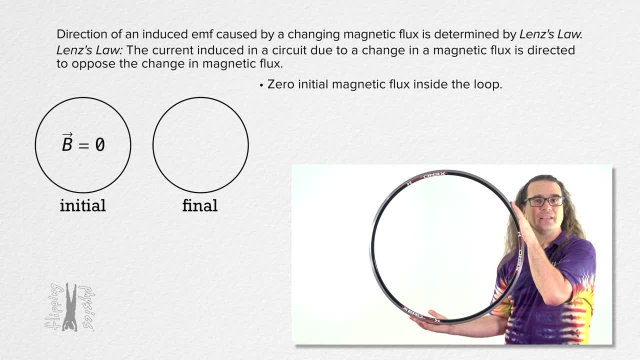 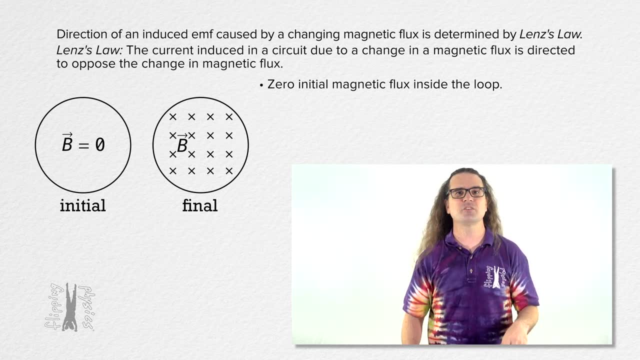 Oh, I see. Okay, Cool, Let's do it. Okay, Here we go. Here we go. magnetic flux inside the loop. Finally, there is a magnetic field into the screen. Remember, the induced EMF and induced current are caused by the change in the magnetic flux. 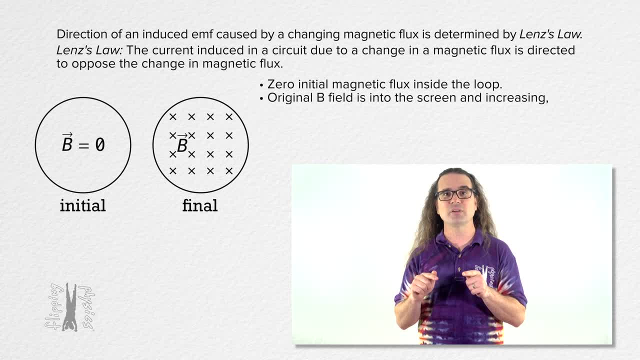 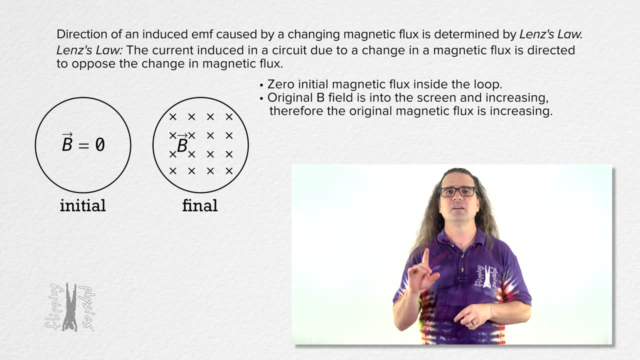 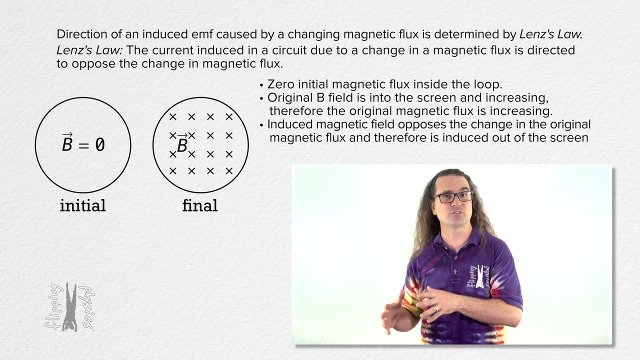 so the original magnetic field inside the loop is into the screen and increasing. therefore the original magnetic flux inside the loop is increasing. According to Lenz's Law, the induced magnetic field opposes the change in the magnetic flux and therefore there is an induced magnetic field out of the screen. 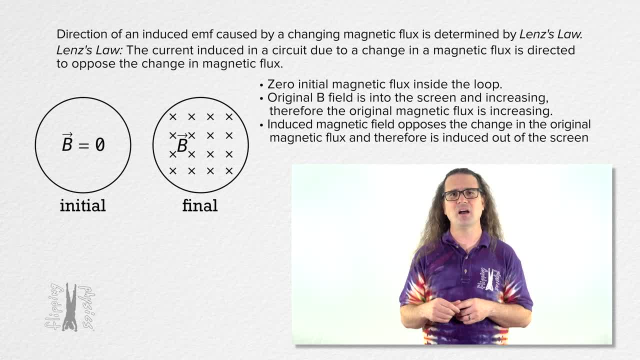 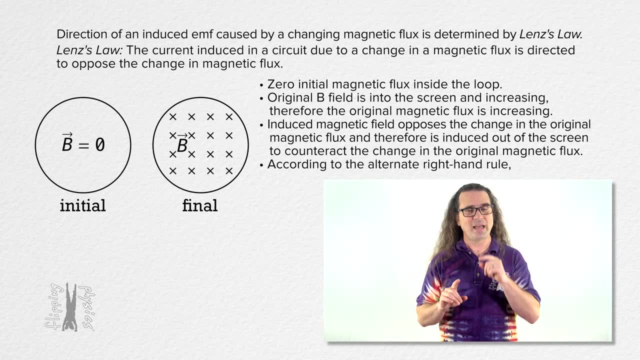 The induced magnetic field is out of the screen because, according to Lenz's Law, it is counteracting the change in the original magnetic flux, which is increasing According to the Right Hand Rule – actually it is the alternate Right Hand Rule, with the thumb pointing in the direction of the induced current. 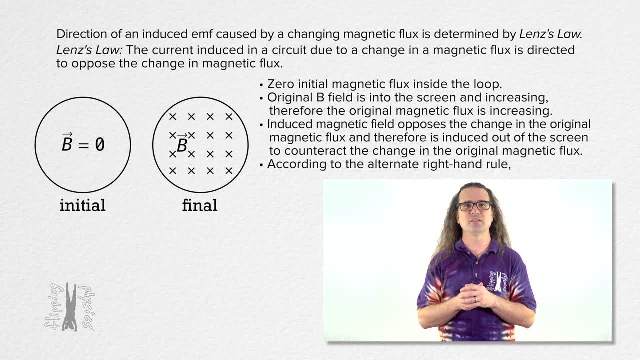 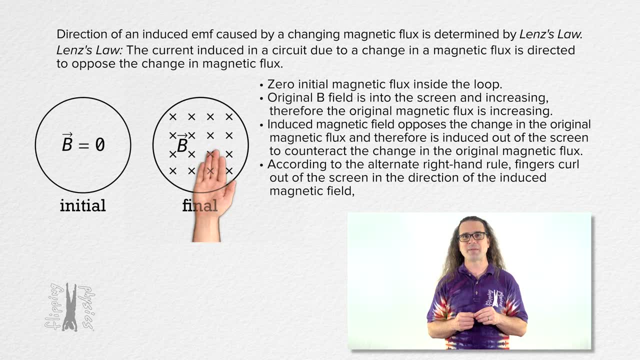 in the wire and the fingers curling in the direction of the induced magnetic field created by the induced current in the wire. so, according to the Right Hand Rule, fingers on the right hand curl in the direction of the induced magnetic field which is out of the screen in the wire loop. 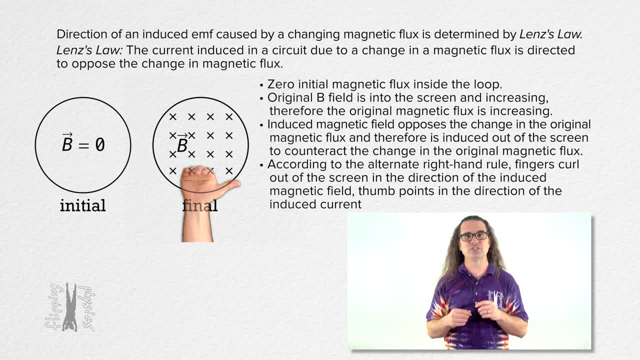 and the thumb of the right hand points in the direction of the induced current in the loop, which makes the induced current in the loop in this example counterclockwise. from this perspective, Again, the induced magnetic field is out of the screen, caused by an induced current in the wire. 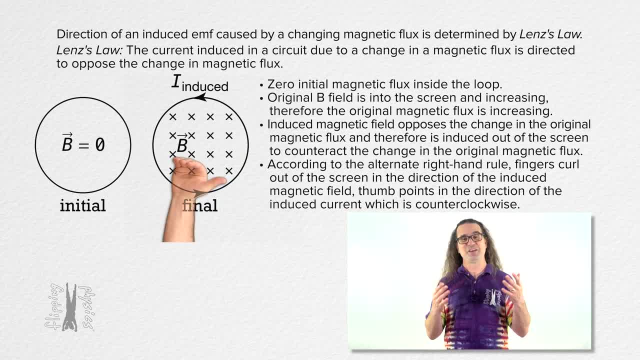 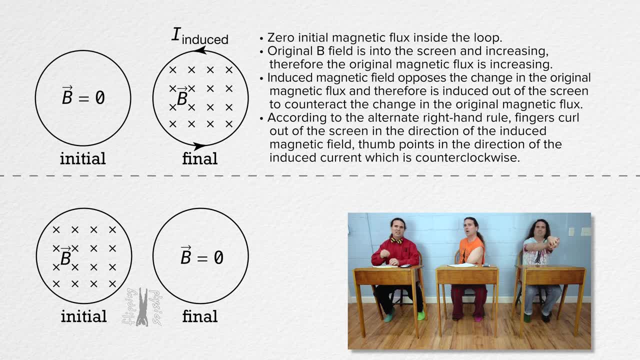 loop which is counterclockwise from this perspective. Okay, that is our first example. Billy, please walk us through our second example. Okay, it looks like the original magnetic field in the loop is into the screen and there is zero final magnetic field, so the original magnetic 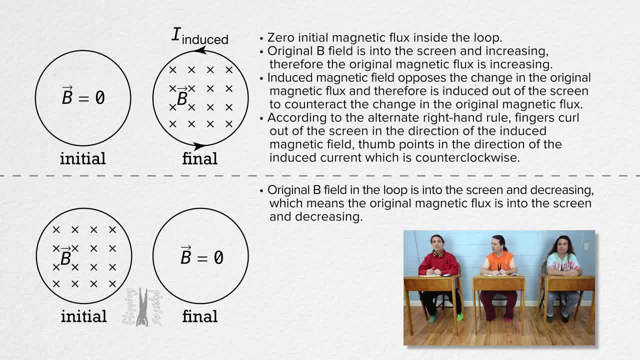 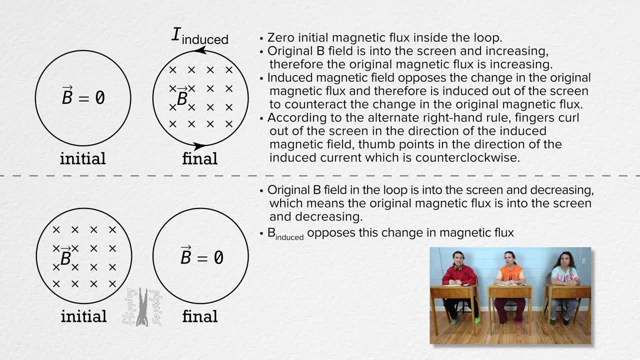 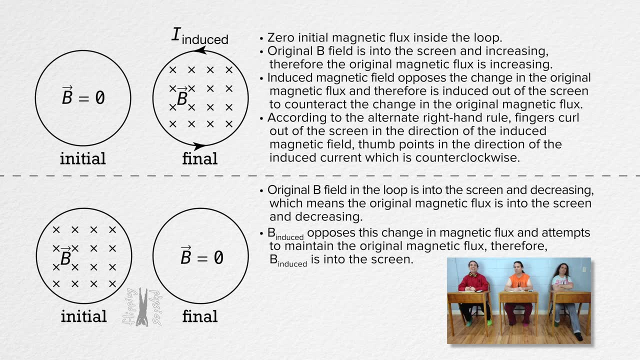 field is into the screen and decreasing, which means the original magnetic flux is into the screen and decreasing The induced magnetic field opposes the change in the magnetic flux. The induced magnetic field attempts to maintain the original magnetic flux, so the induced magnetic field is into the screen. I thought magnetic flux was a scalar. How can the original magnetic flux 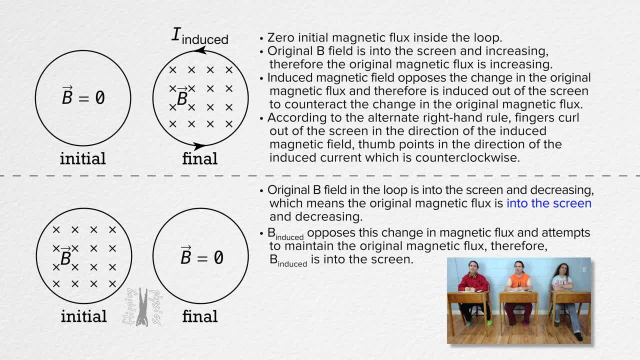 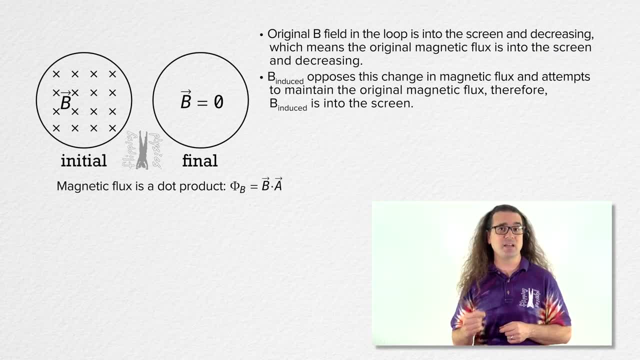 be equal into the screen if it is a scalar and does not have direction. Good point, Bobby. This is a common point of confusion. Magnetic flux is a dot product, so magnetic flux is a scalar. So the induced magnetic flux does not have a direction. However, 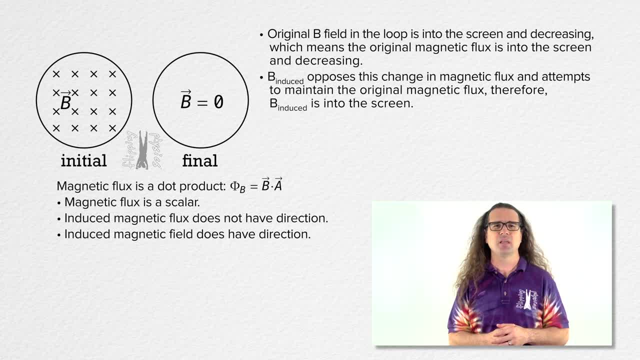 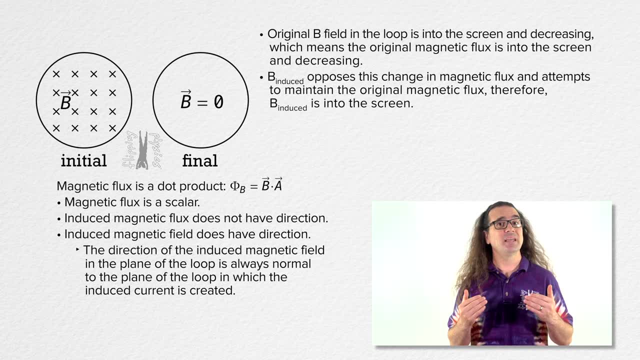 the induced magnetic field does have a direction, And the direction of the induced magnetic field in the plane of the loop is always normal to the plane of the loop in which the induced current is created. Got it? The induced magnetic field in the plane of the loop is always normal to the loop. 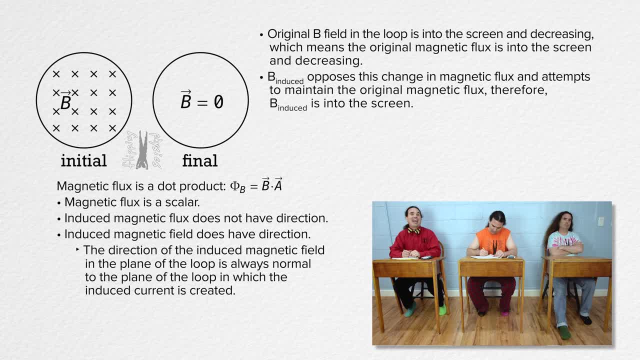 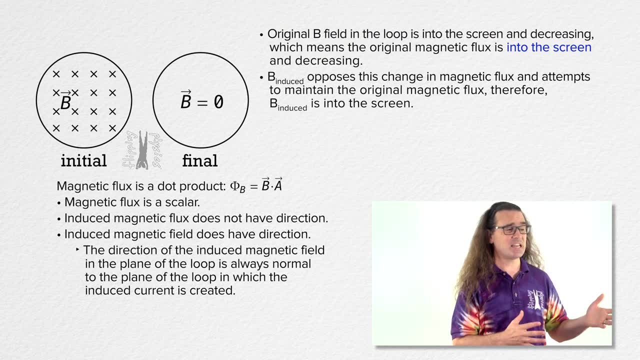 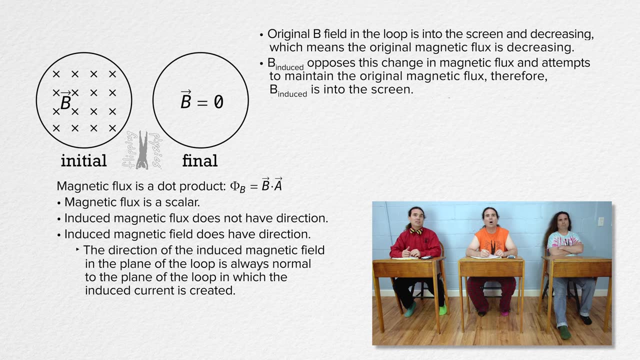 in which the induced current is created. Thanks. So please, Billy, start back at the beginning of this example and remember magnetic flux is a scalar and does not have direction. Certainly The original magnetic field in the loop is into the screen and decreasing The induced magnetic. 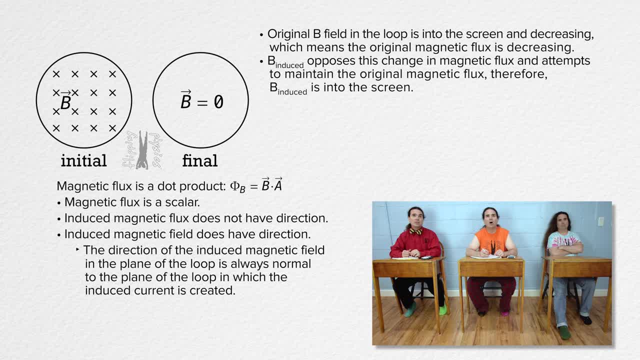 field opposes that change in the magnetic flux. so the induced magnetic field is into the screen to try to change the magnetic flux. So if the induced magnetic field is in the loop, the keep the magnetic flux constant And the direction of the induced current in the loop. 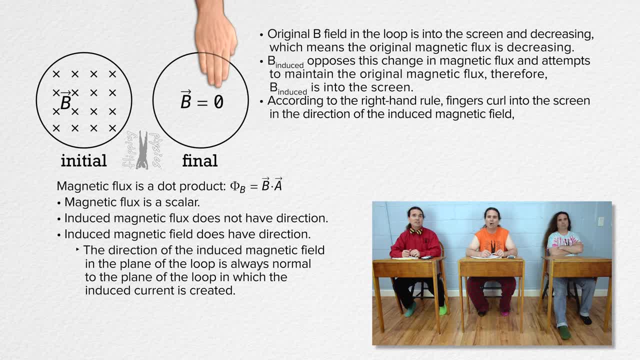 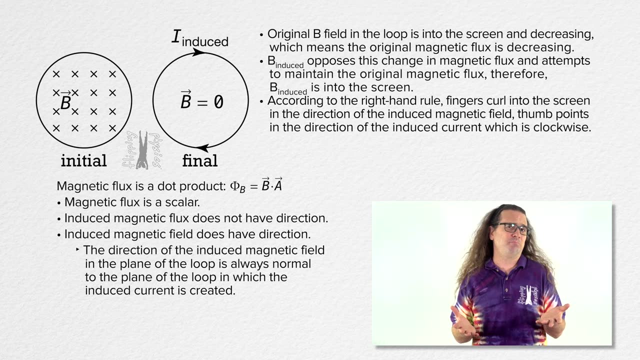 According to the alternate right-hand rule, the fingers curl in the direction of the induced magnetic field, which is into the screen, thumb points in the direction of the induced current, which is clockwise. from this perspective, That is a lot, Yeah, Yeah, it kinda is. 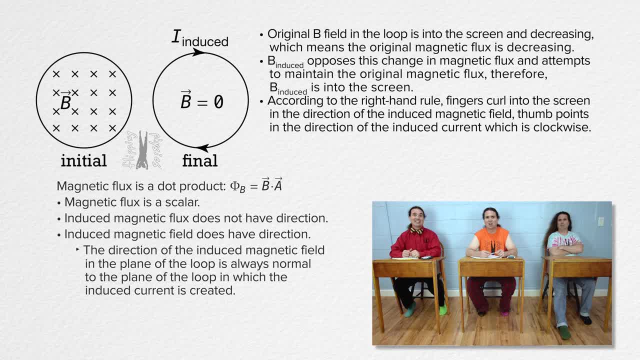 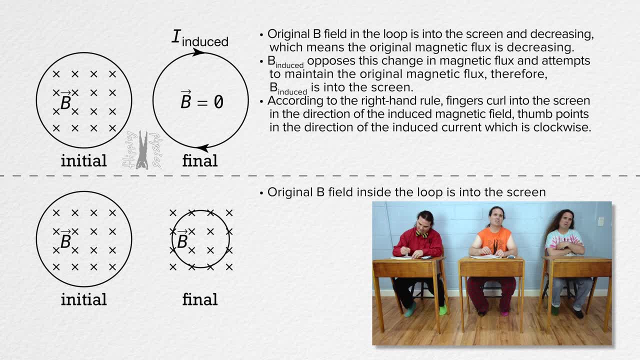 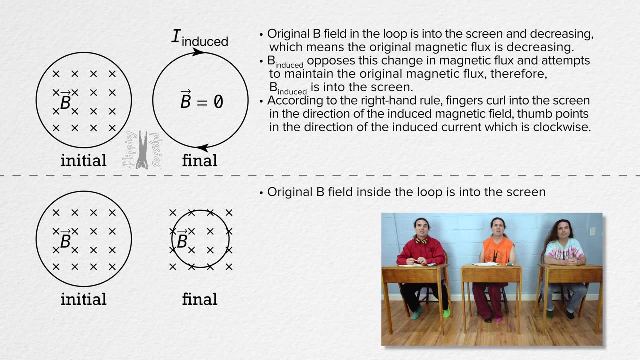 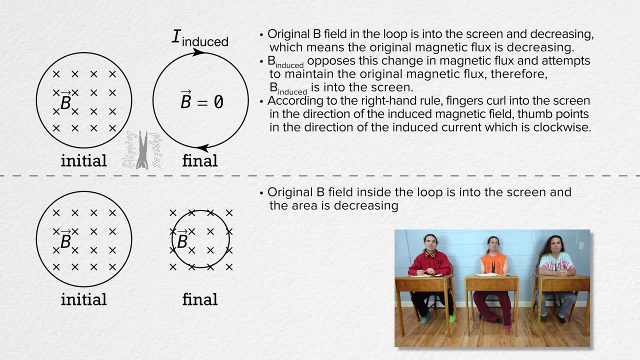 but it's also pretty cool. Yeah, Sure, Okay, Bobby, please walk through the next example. Okay, Initially, the magnetic field inside the loop is into the screen. The magnetic field is the same direction at the final point, but the area of the loop has decreased. Okay, so because the area of the loop is decreasing, 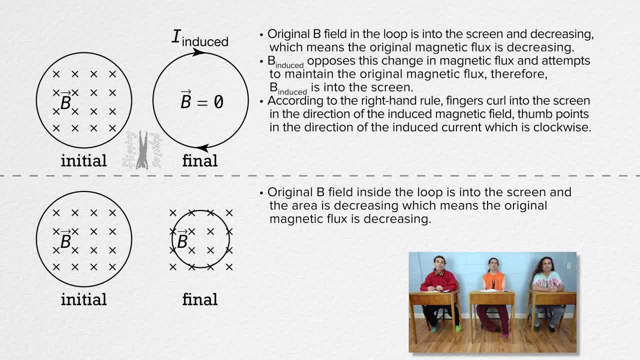 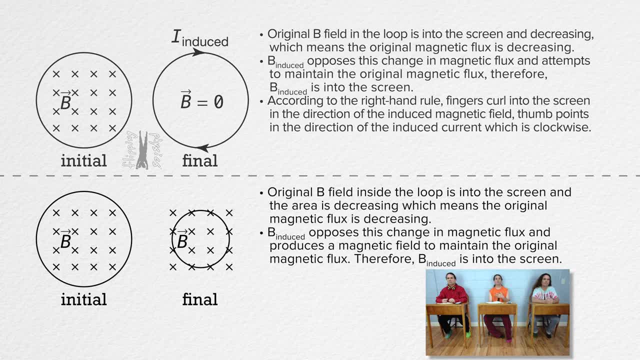 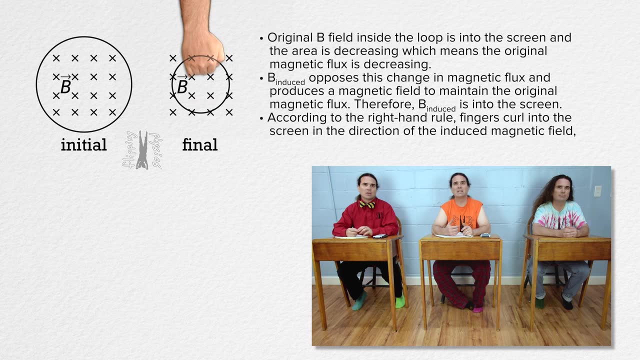 the magnetic flux through the loop is decreasing, The induced magnetic field opposes that change in magnetic flux. so the induced magnetic field is into the screen. The magnetic field is into the screen to attempt to maintain the original magnetic flux According to the right-hand rule. the fingers curl into the screen in the direction of the. 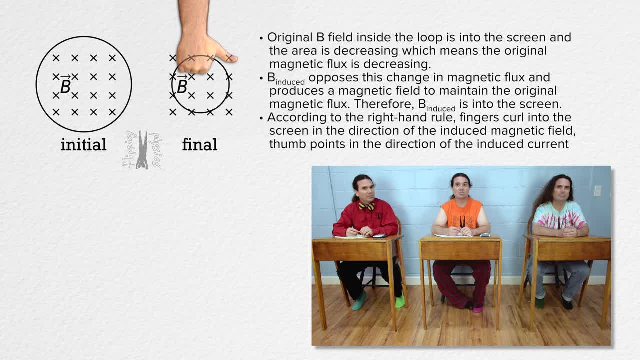 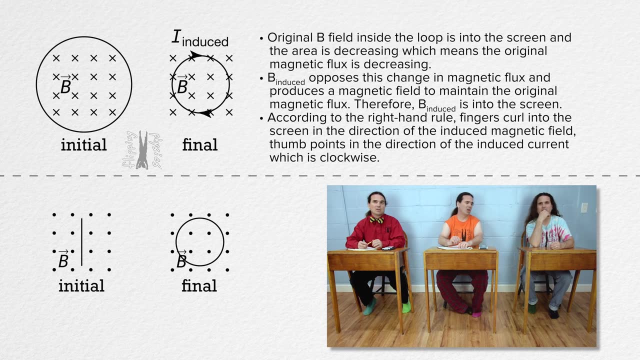 induced magnetic field thumb points in the direction of the induced current, which is clockwise from this perspective. The induced current, from this perspective, is clockwise. Very nice, Bobby Bo, please do the next one. Sure, But I don't really get the illustration. What am I looking at? Initially, the loop is not a magnetic field. See, like the current leads to the magnetic field, but the inducing current from the Induced magnetic field is not And the induction current is not, Though the magnetic field is in the direction of the current, so the inducing current is not. 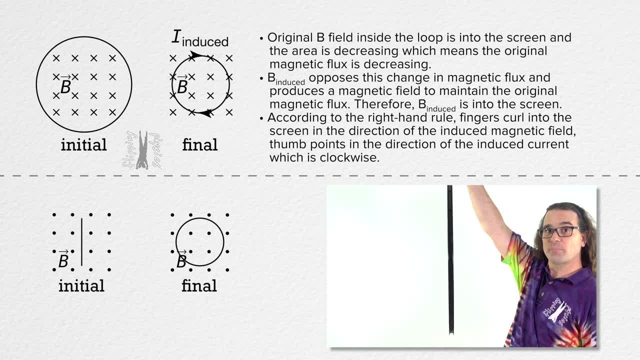 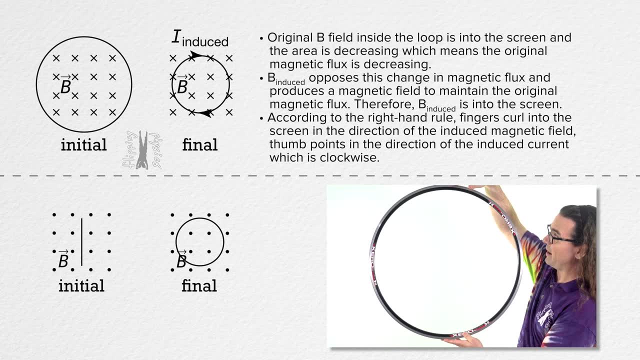 normal, to the plane of the screen. so all you can see is the profile of the loop. Then the wire loop is turned such that at the final point the loop is parallel to the screen. Got it Thanks. Initially the magnetic field is out of the screen. 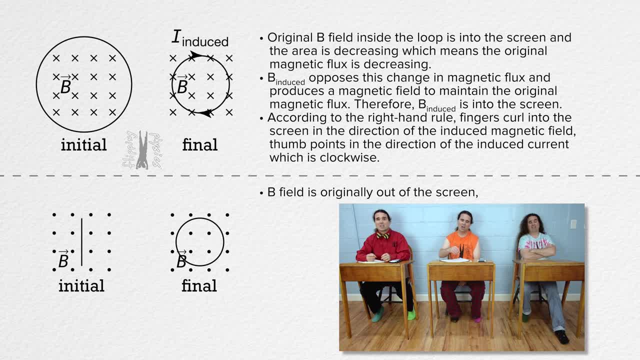 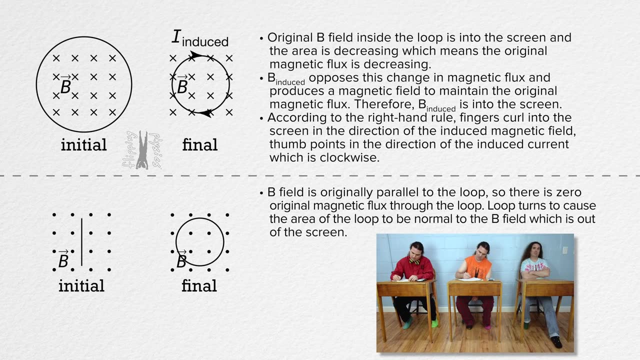 but what we are really interested in is the initial magnetic flux. Initially the magnetic field is parallel to the wire loop, so zero magnetic field lines pass through the loop. so initially there is zero original magnetic flux. The loop is turned so that at the final point the magnetic field is out of the screen and passing through the loop. 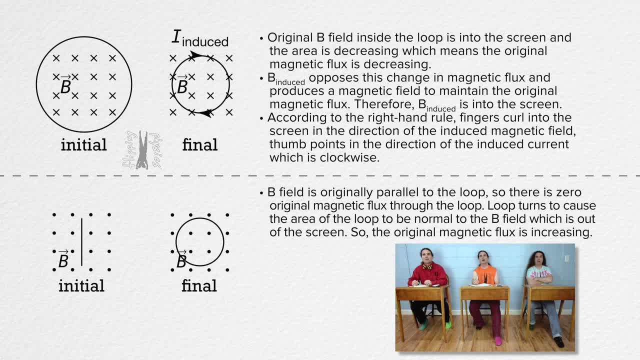 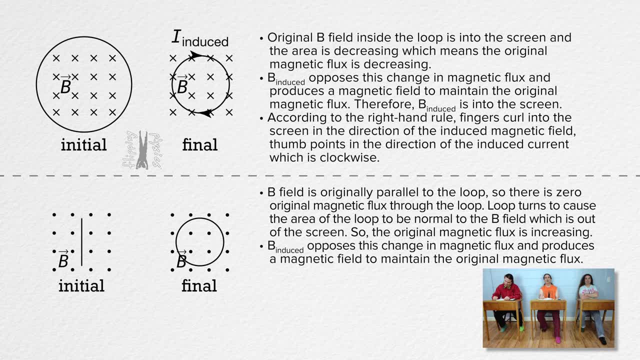 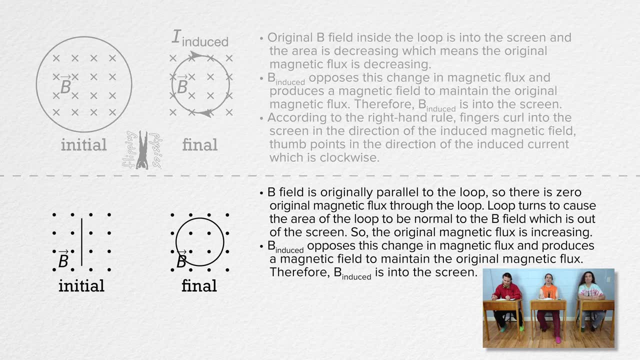 so the original magnetic flux is increasing in magnitude. That means the induced magnetic field is opposite the direction of the original magnetic field to try to maintain a constant magnetic flux through the loop. So the induced magnetic field through the loop is into the screen. 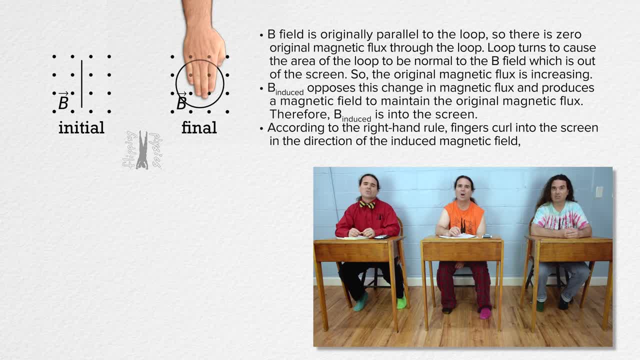 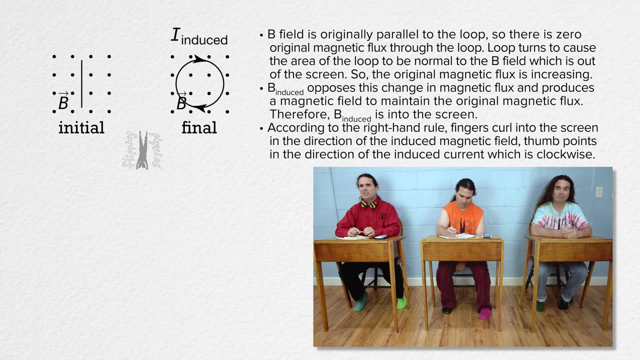 Using our right hand, we curl our fingers into the screen and our thumb points, clockwise from this perspective, in the direction of the current induced in the wire. Yeah, the induced current is clockwise from this perspective, But which way did you rotate the loop? 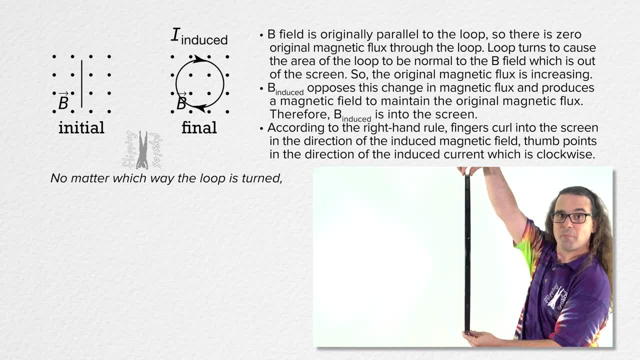 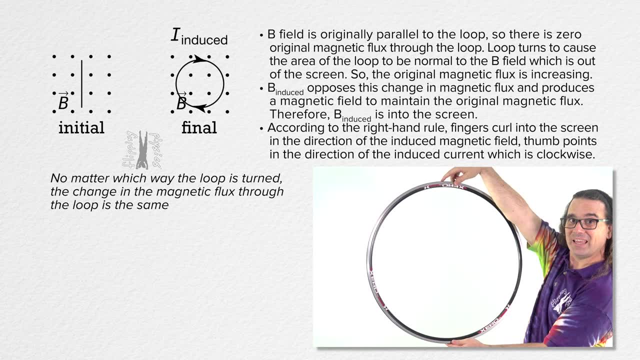 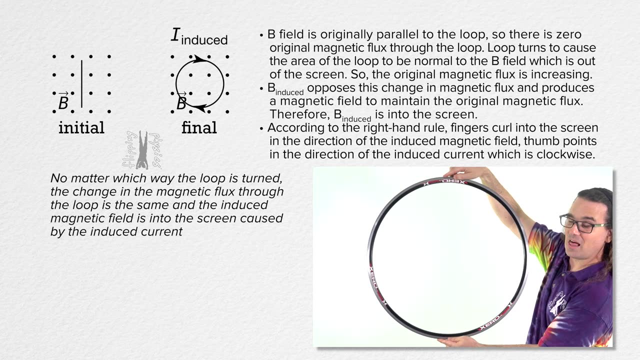 Yes, Billy. thanks. Notice that no matter which way I turn the loop, the change in the magnetic flux through the loop is the same and the induced magnetic field is into the screen caused by the induced current, which is clockwise. from this perspective, That is strange. It does not matter which way you rotate the loop. 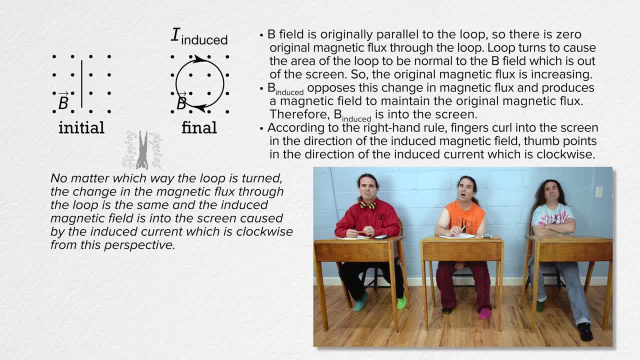 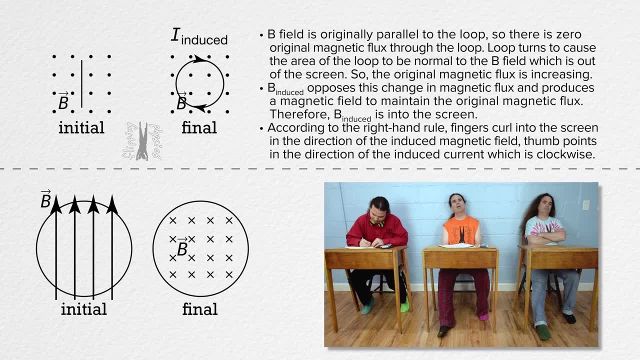 The induced current will always be clockwise from this perspective. Okay, I guess sometimes physics is strange. Yes, Billy, Bobby, please do this one. Okay, the original magnetic flux is in the direction of the current induced in the wire. The original magnetic field is parallel to the loop initially. 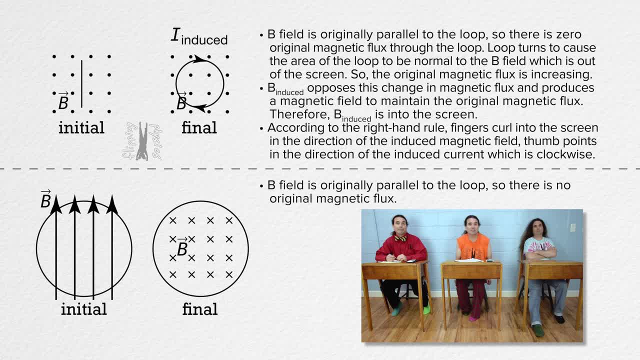 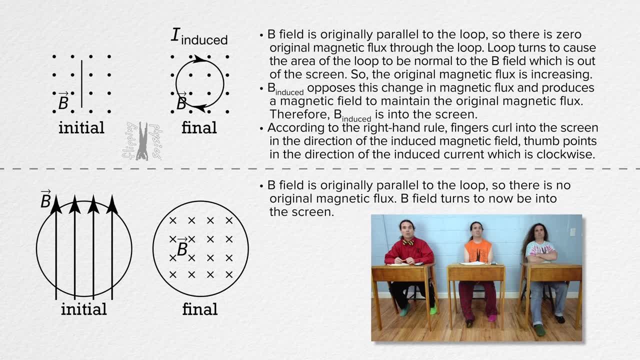 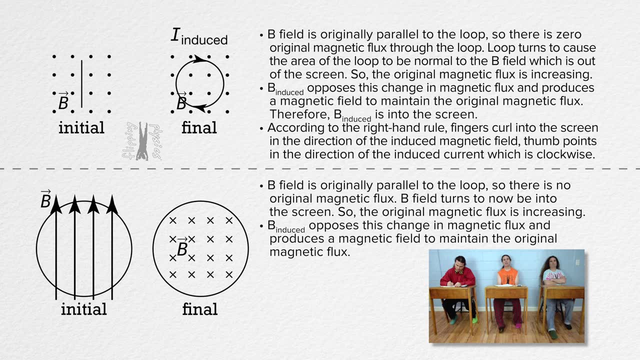 That means initially there is zero original magnetic flux through the loop. The magnetic field then turns and at the final point is into the screen. So the original magnetic flux is increasing. The induced magnetic field opposes this changing magnetic flux, so it produces a magnetic field which is out of the screen. 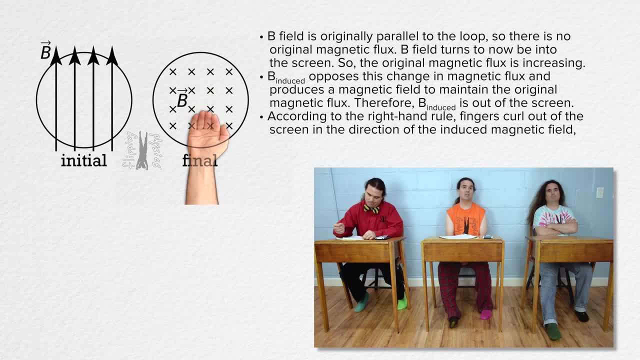 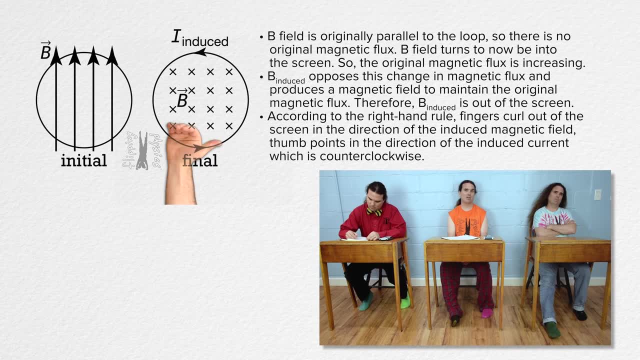 According to the right-hand rule, fingers curl out of the screen in the direction of the induced magnetic field and thumb points in the direction of the induced current in the loop, which is counterclockwise from this perspective If the magnetic field is changing directions. 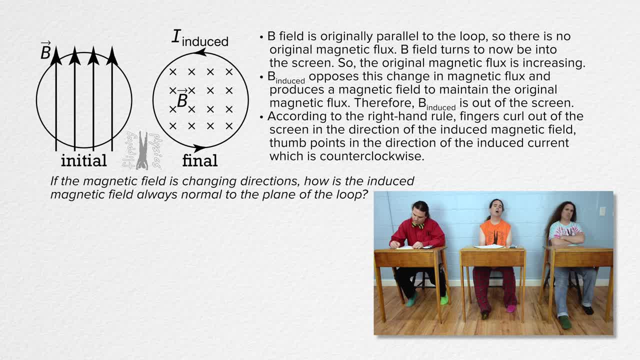 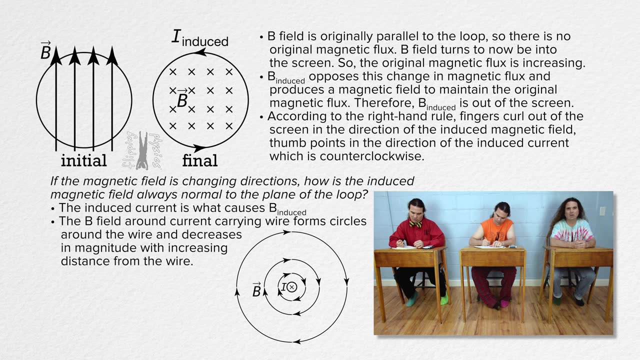 how is the induced magnetic field always normal to the plane of the loop? The induced current is what causes the induced magnetic field. In a previous lesson we showed that the magnetic field around a current carrying wire forms circles around the wire and decreases in magnitude as distance from the wire increases. 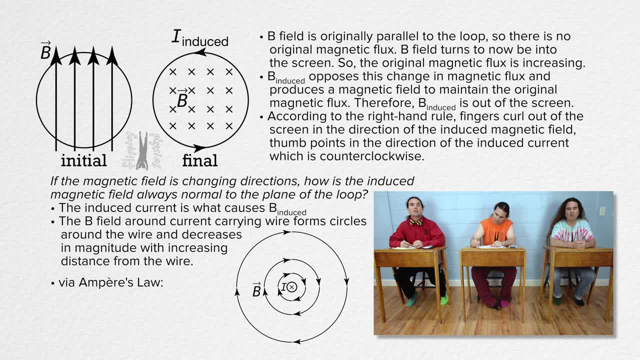 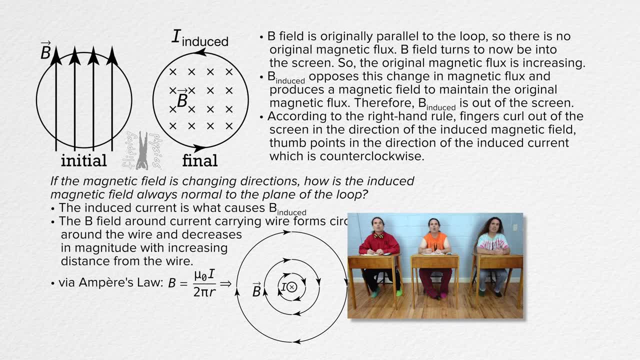 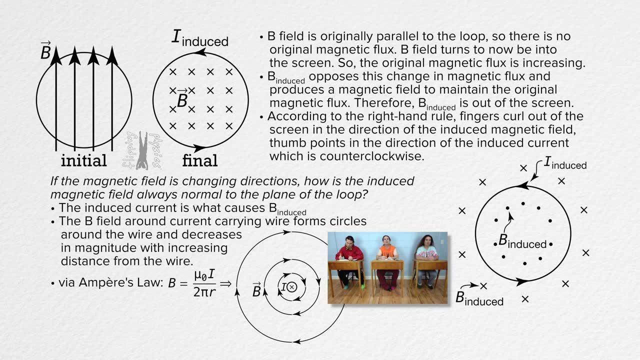 We even used Ampere's law to derive the equation for the magnitude of the magnetic field around a current carrying wire. Okay, I get it. The induced magnetic field is only normal to the plane of the loop in the plane of the loop. In locations outside the plane of the loop, the magnetic field is sort of in the shape of a torus. 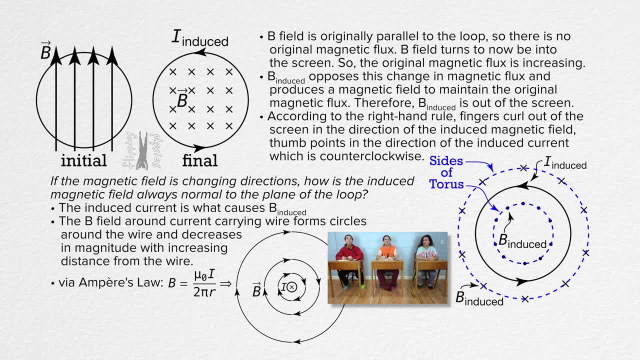 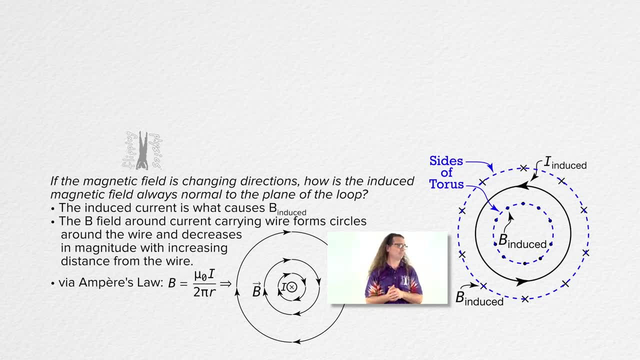 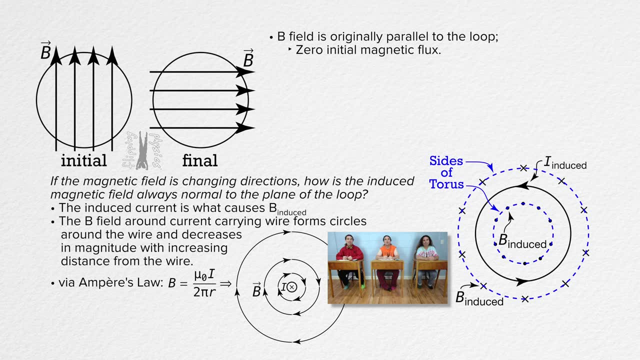 Torus. What is a torus? A doughnut? Oh Yes, thank you. That is a great explanation, Billy. please explain this last example Certainly: Initially the magnetic field is in the plane of the loop, so zero field lines pass through the loop and there is zero initial original magnetic flux. 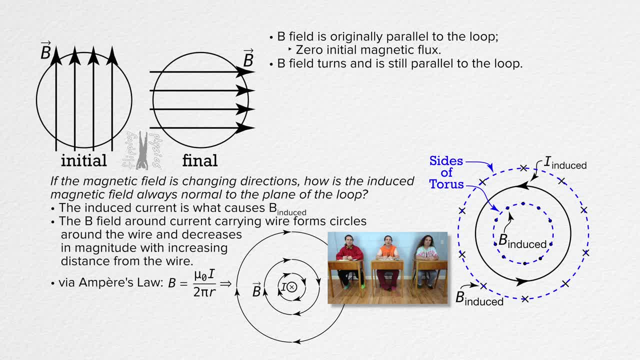 The magnetic field turns 90 degrees, but the final magnetic field is also in the plane of the loop and therefore the final magnetic flux is also zero. Therefore there is no change in the magnetic field. There is no change in the magnetic flux in this example. 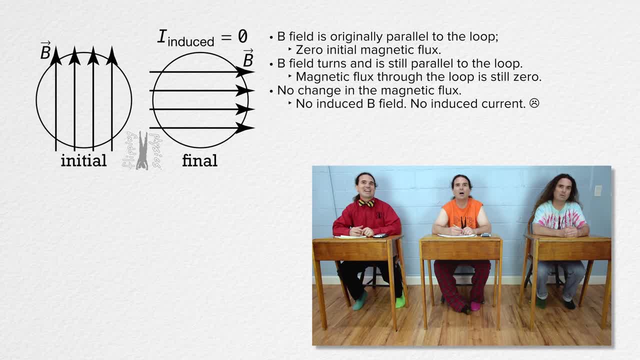 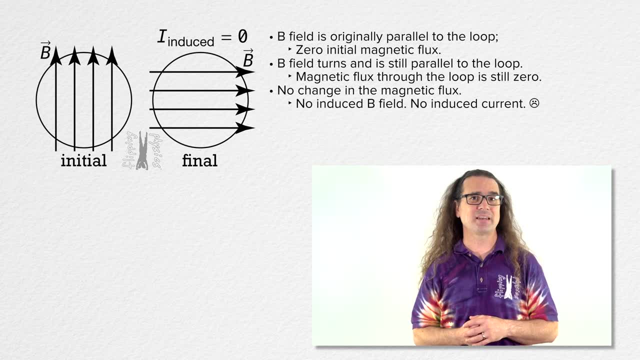 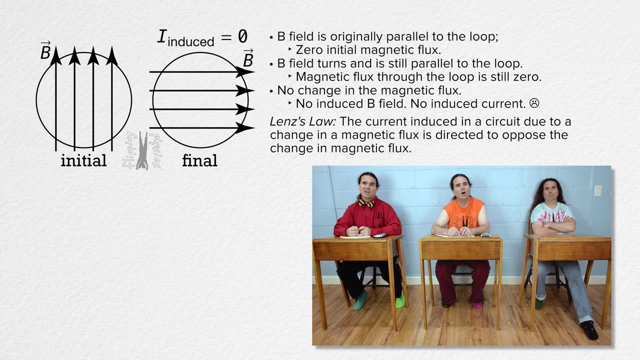 so there is no induced magnetic field and no induced current in the wire. Absolutely Billy. when there is no change in the magnetic flux in the loop, there is no induced magnetic field, even if the magnetic field is changing directions. I hope that helps clear up Lenz's law, which describes the direction of the induced current. 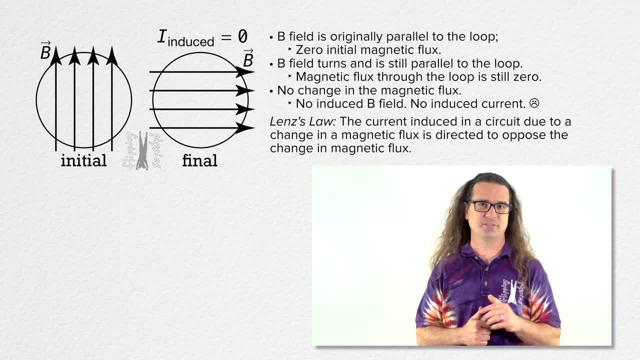 in a loop which is created by a changing magnetic flux. At this point, we have covered all four of Maxwell's equations. At this point, we have covered all four of Maxwell's equations. At this point, we have covered all four of Maxwell's equations. 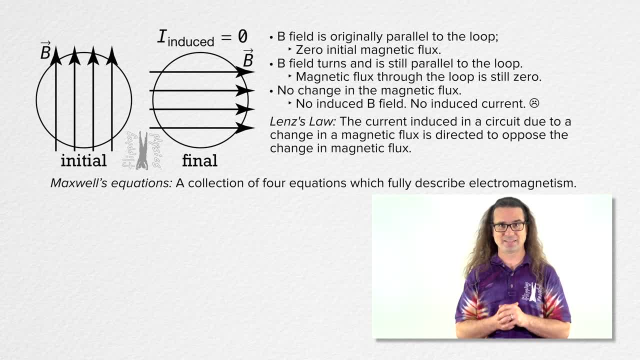 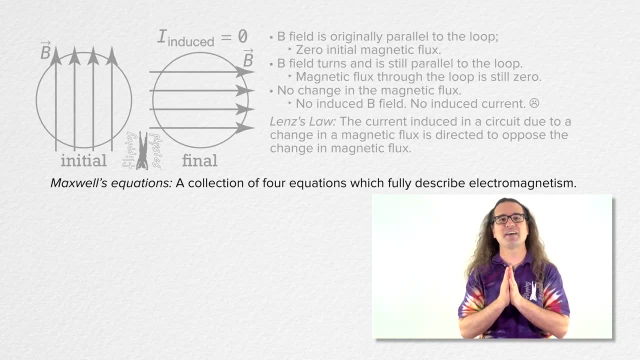 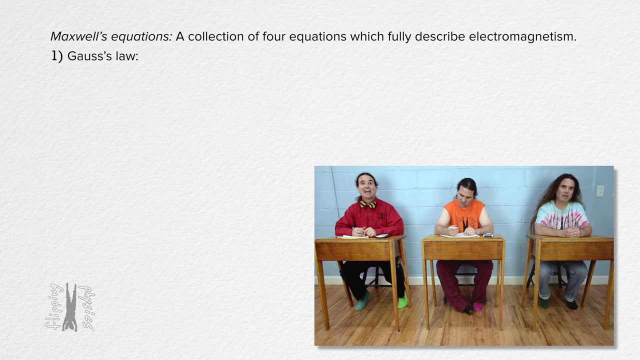 which are a collection of equations which fully describe electromagnetism. So let's specifically identify all four of them. The first one is Gauss's law. Bo, remind me what is Gauss's law? Gauss's law states that the electric flux through a closed surface equals the closed surface integral. 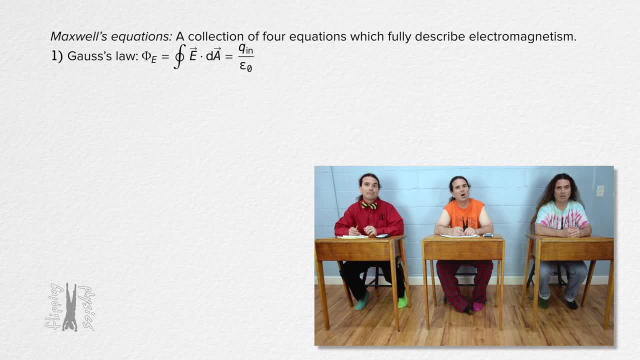 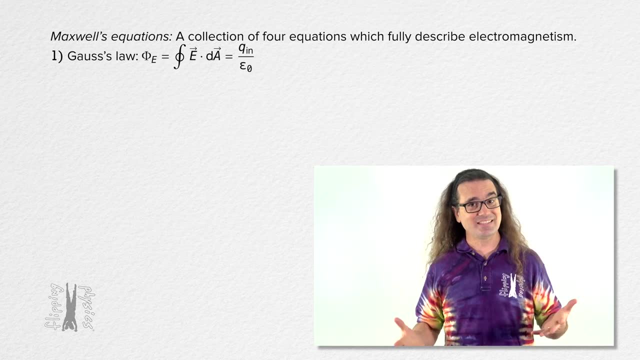 of the dot product of electric field and area dA, which equals the charge enclosed in the Gaussian surface divided by the permittivity of free space. Thank you, Bo. As I said, the first of Maxwell's equations is called Gauss's law. 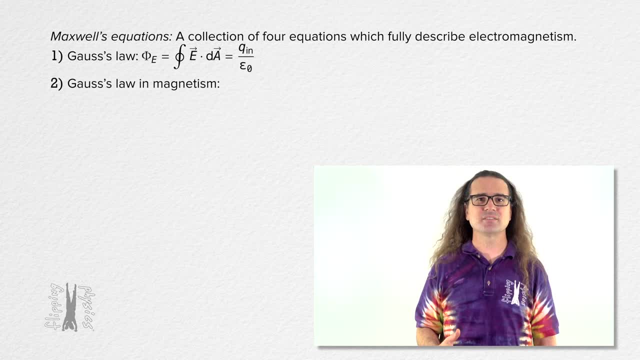 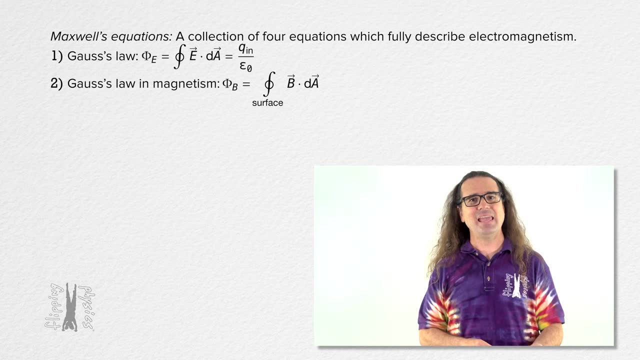 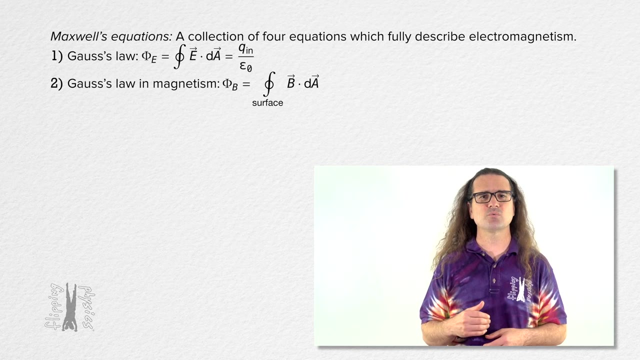 The second of Maxwell's equations is Gauss's law in magnetism, which is very similar to Gauss's law, only it deals with magnetic flux and magnetic field. And because all magnetic field lines are loops, the number of magnetic field lines which go into and out of a closed surface will be the same, meaning the magnetic flux through a closed 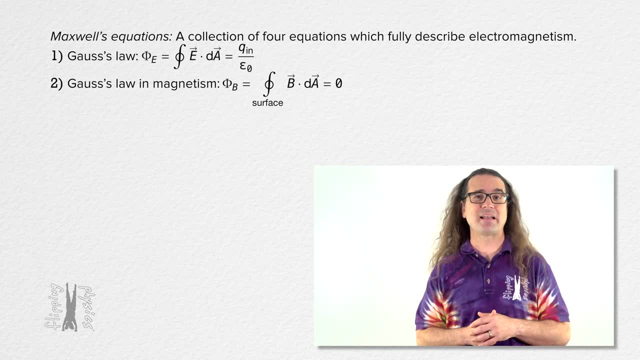 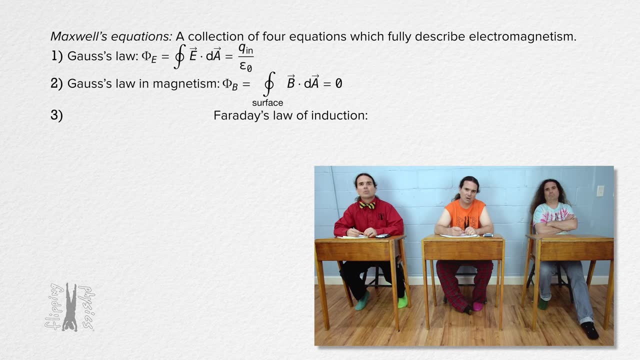 surface will always equal zero. The third of Maxwell's equations begins with Faraday's law of induction. Bobby, what is Faraday's law of induction? Faraday's law of induction states that induced EMF equals the negative of the derivative of magnetic flux with respect to time. 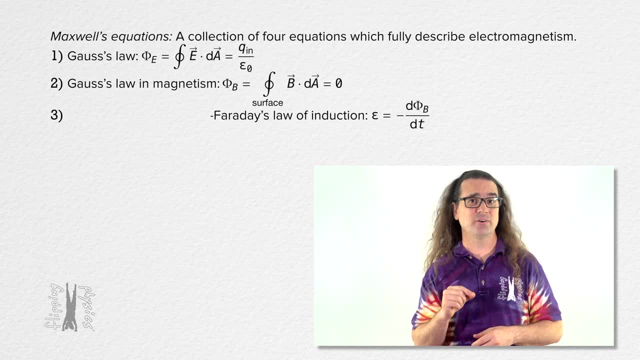 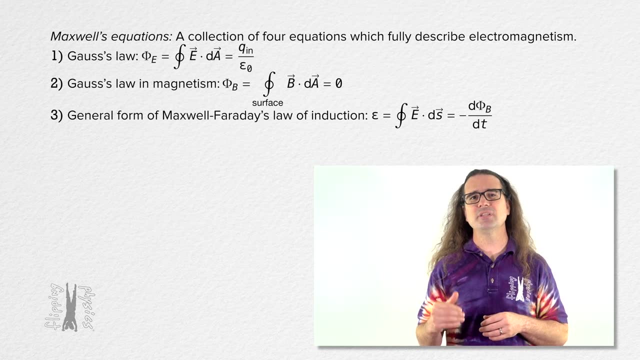 Correct. However, Maxwell's third equation is a more general equation and is often called the general form of Maxwell-Faraday's law of induction. It states that the induced EMF equals the closed loop integral of the dot product of the electric field and the infinitesimal distance ds, which equals the negative of the derivative of the. 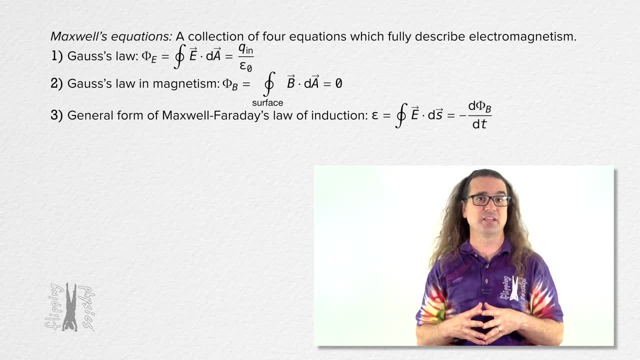 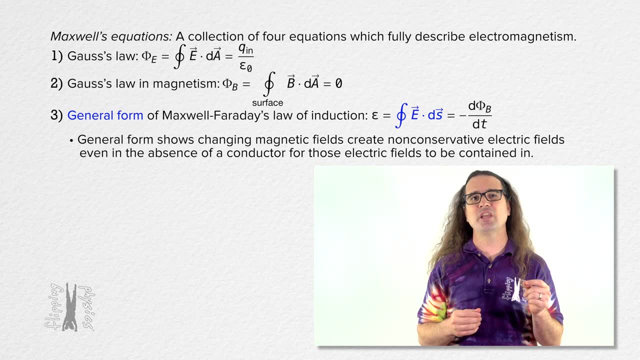 magnetic flux with respect to time or the time rate of change of the magnetic flux. The more general equation adds the middle part of the equation, which shows that the changing magnetic fields create non-conservative electric fields even in the absence of a conductor for those electric fields to be contained in. 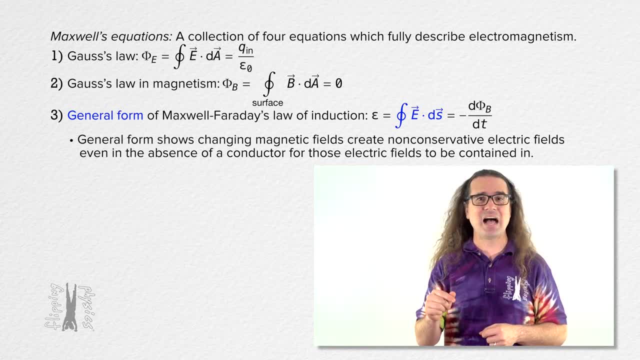 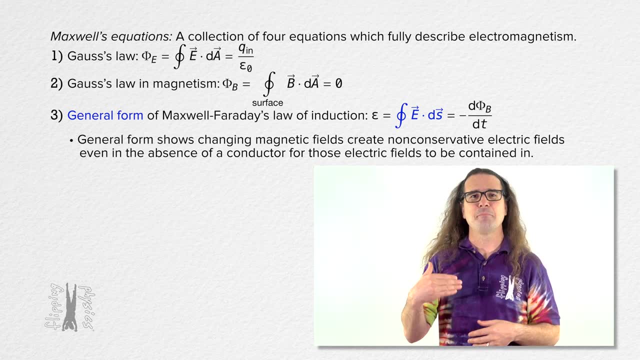 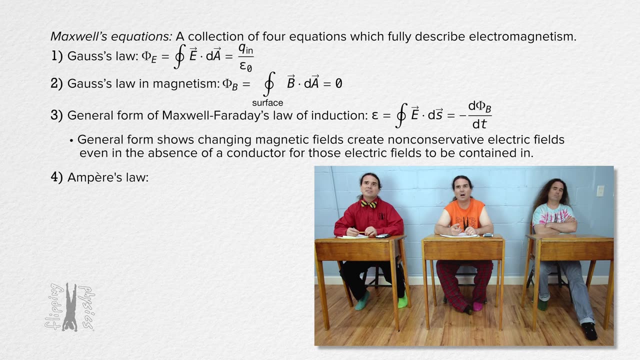 That's right. A changing magnetic flux creates non-conservative electric fields in free space, No electrical conductor needed. And Maxwell's fourth equation begins with Ampere's law. Billy, what is Ampere's law? Ampere's law states that the closed loop, integral of the dot, product of the magnetic field and the 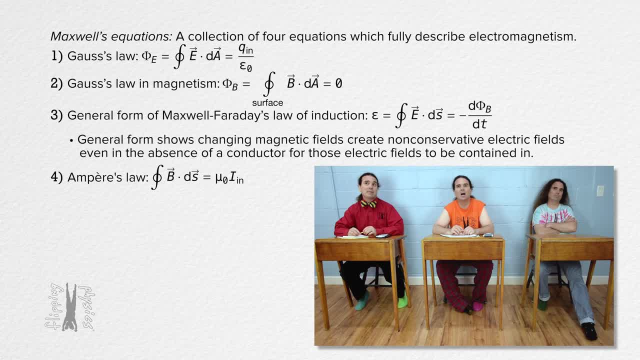 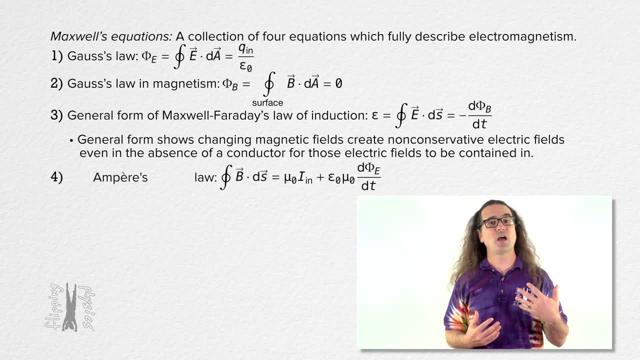 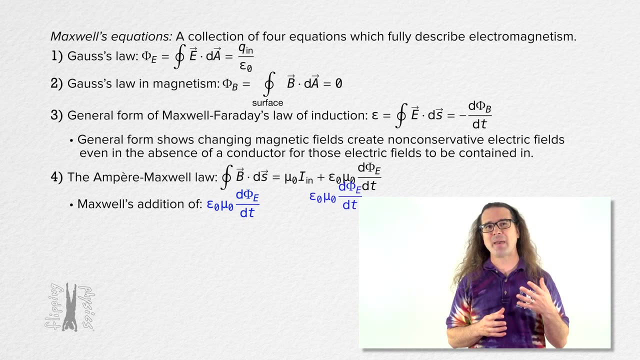 infinitesimal distance. ds equals the magnetic permeability of free space times, the current through the plane of the amperian loop. Correct. Billy Maxwell's fourth equation is called the Ampere-Maxwell law and adds the following to Ampere's law: Electric permittivity of free space times. magnetic permeability of free 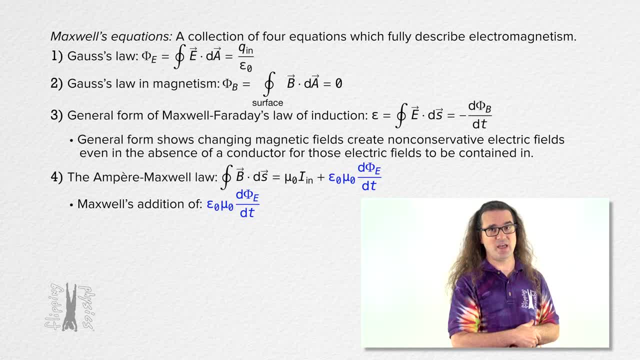 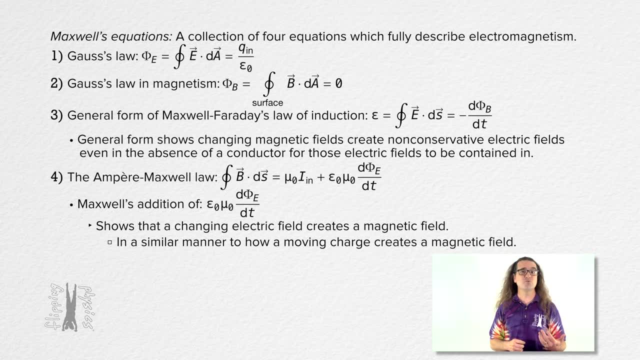 space times, the derivative of electric flux with respect to time. This shows that a changing electric field creates a magnetic field in a similar manner to how a moving charge creates a magnetic field. So those are all four of Maxwell's equations, Mr P. 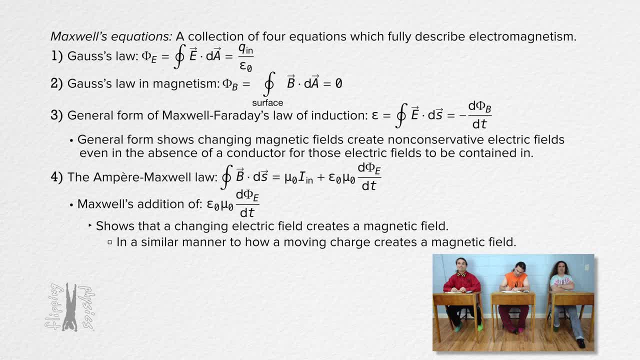 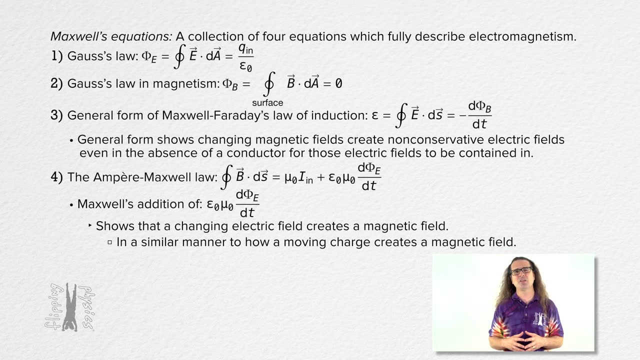 Yes, Bo, Why are those four equations called Maxwell's equations if they have so many other names in them as well? I mean, the first two don't even have Maxwell's name in them, right? That is a fair question, Bo, And the truth is that the naming of laws can be quite 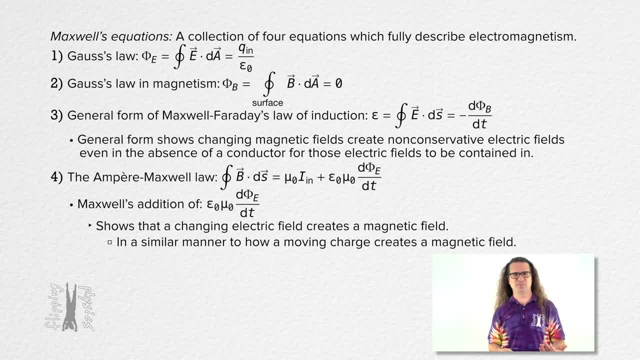 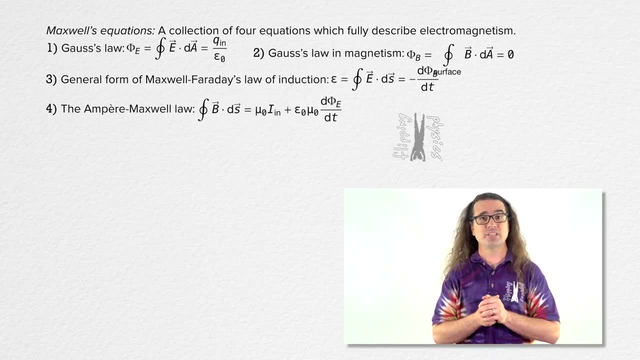 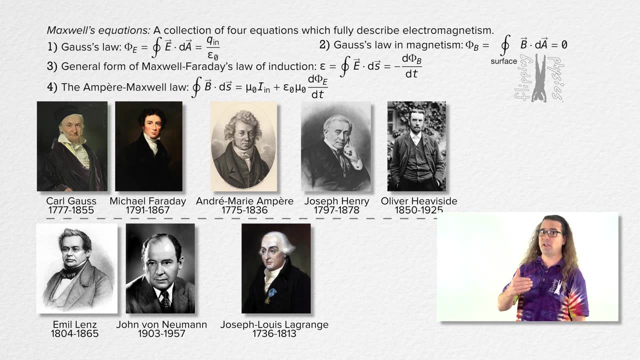 complicated And there can be a lot of politics involved. There are many scientists responsible for discovering Maxwell's four equations, which fully describe electromagnetism, For example Gauss, Faraday, Ampere, Henry, Heaviside, Lentz, Newman, Lagrange, Maxwell and honestly. 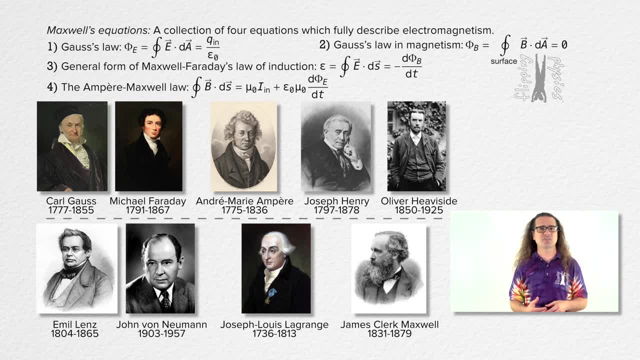 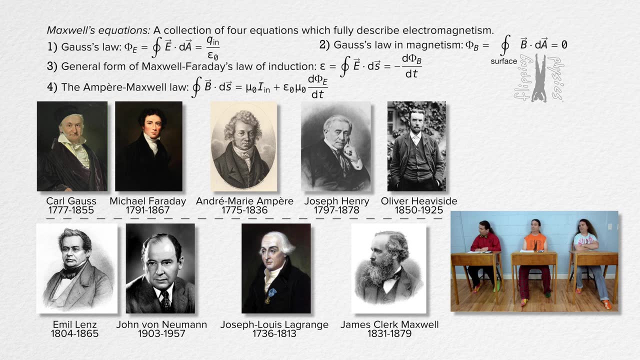 probably more. In the end, Maxwell gets credit for having contributed significantly to the discovery of these equations and identifying that combined they fully describe electromagnetism. Basically, we call them Maxwell's equations. however, recognize that there are a lot of people. 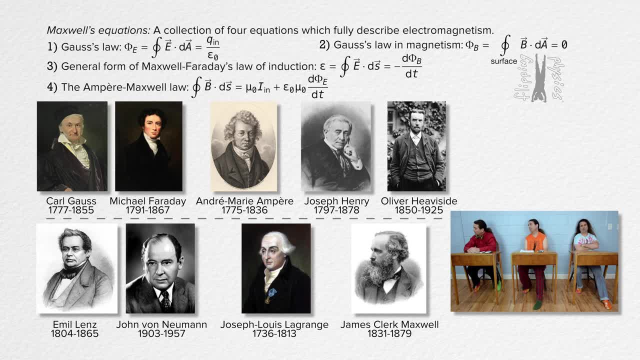 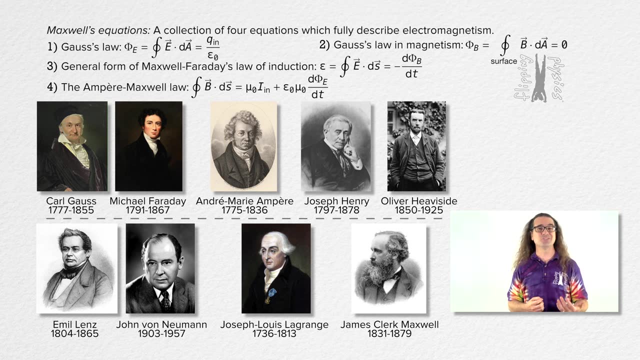 who contributed to their discovery. I wonder who got to write the history books. I know I think we're looking at them right now. Yeah, That concludes my review of electromagnetic induction for AP Physics C: Electricity and Magnetism. Next time we are going to review induced forces. 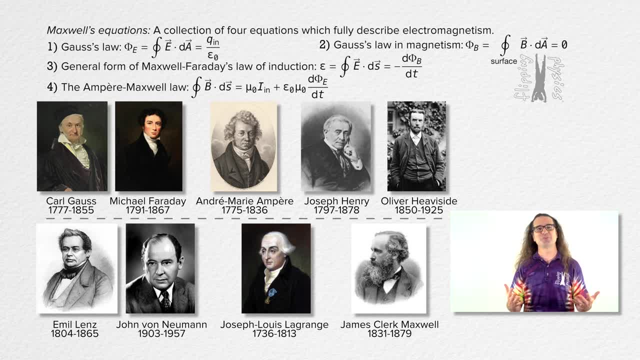 Thank you very much for learning with me today. I enjoy learning with you. 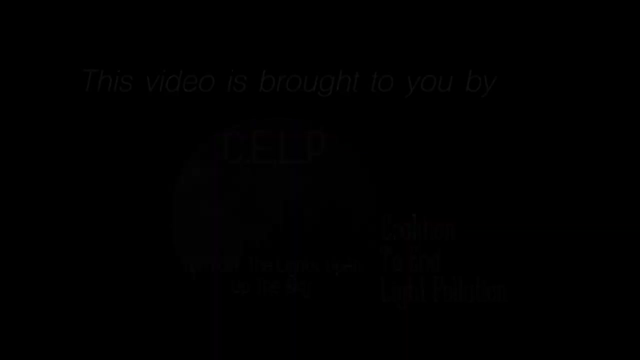 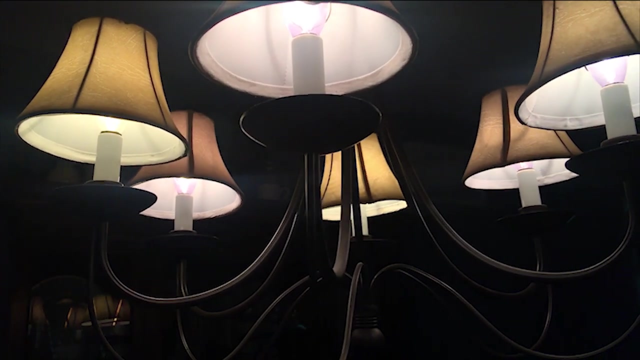 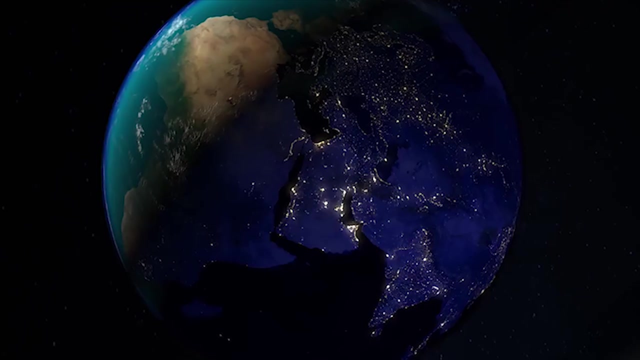 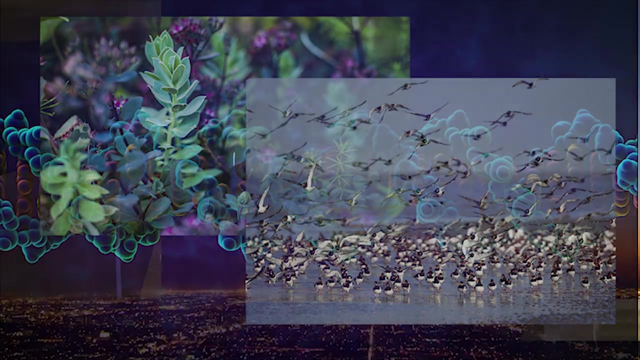 Ever since the light bulb's invention 150 years ago by Thomas Edison, artificial light has illuminated homes, streets and skies, but with some unintended consequences. For billions of years, all life has relied on Earth's predictable cycle of day and night. It's encoded in the DNA of all plants and animals. Humans have radically disrupted.